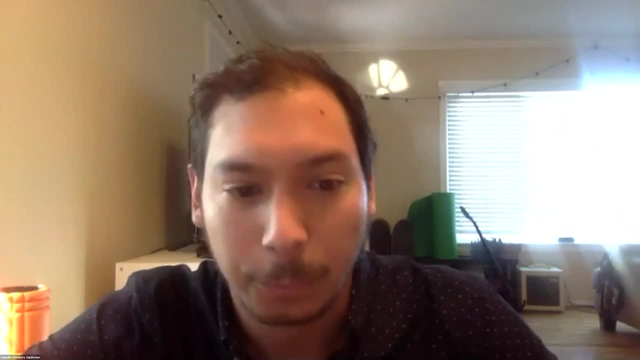 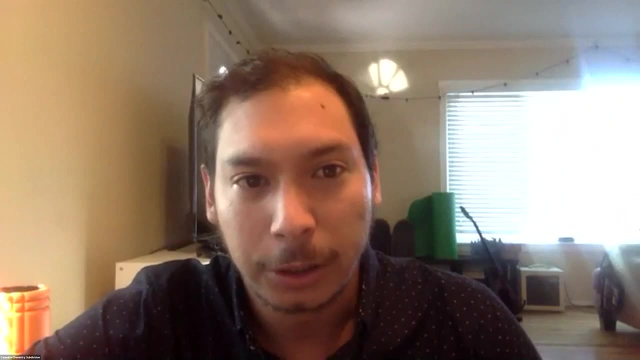 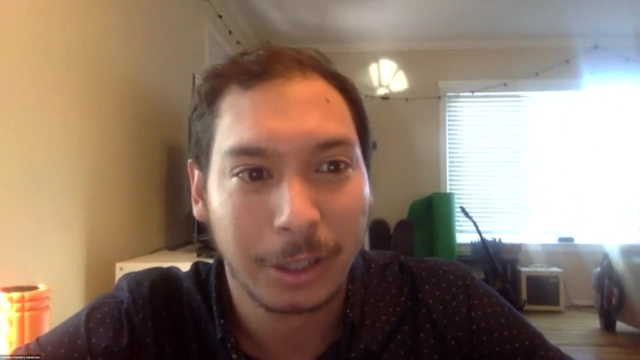 All right, We are a minute after, so we'll go ahead and get this started. Thanks everyone for joining. My name is Kyle Boyer and I'll be your host for today. Welcome to the October edition of Cannes Journal Club. Today, we're going to be discussing heavy metals and cannabis. 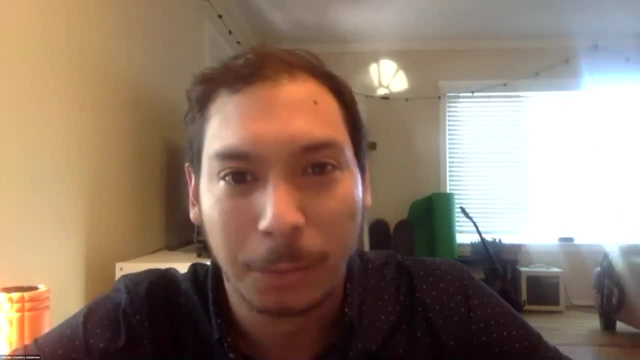 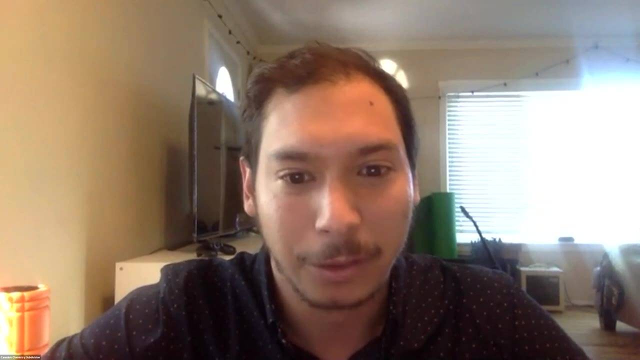 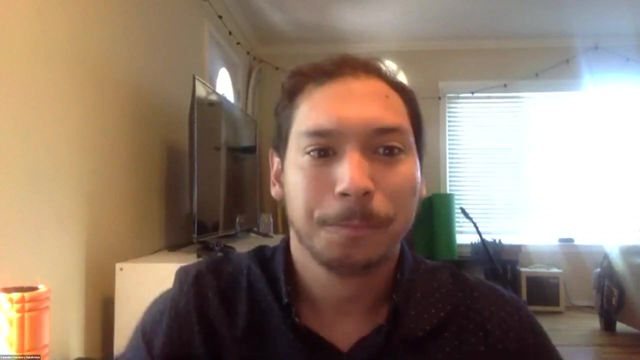 and the latest development in testing protocols, and I'm joined here by Dr Jenny Nelson And she'll be talking about her AOAC first action method, as well as some of her efforts towards developing an ASTM method, and I'll give a little bit about Dr Nelson. So, Dr Nelson- 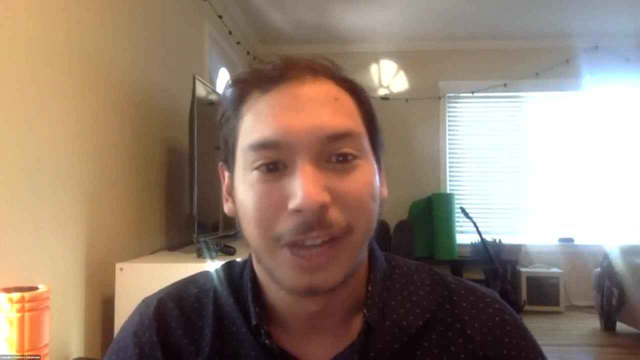 received her PhD in analytical chemistry from the University of Cincinnati in 2007, and her MBA from St Mary's College of California in 2011.. Currently, Jenny is an application scientist at Agilent Technologies and she joined in 2012.. 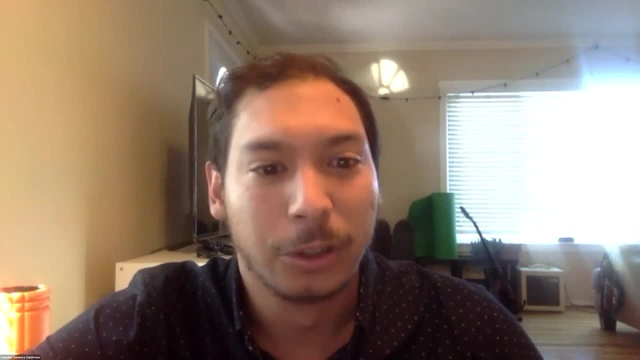 Jenny is also an adjunct professor in the Department of Viticulture and Enology at the University of California Davis since 2013.. She's been very active with AOAC and ASTM over the past eight years, serving on expert review panels, chairing committees and volunteering to develop. 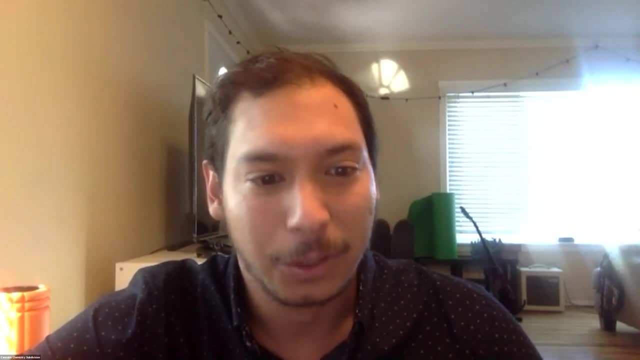 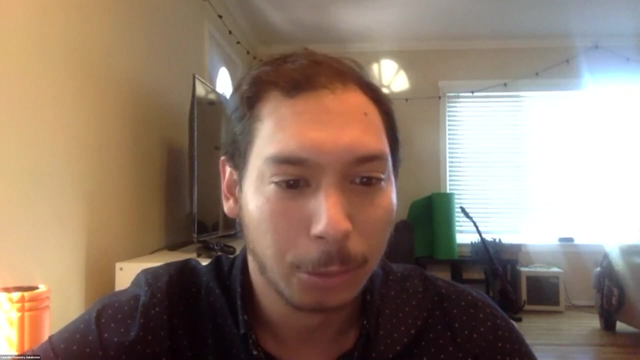 new methods needed by the industry. Jenny has extensive experience in operating and method development for inductively coupled plasma mass spectrometry, ICP-MS, which we'll be talking about today. Inductively coupled plasma- optical emission spectroscopy- so ICP-OES, as well as microwave plasma, atomic emission. 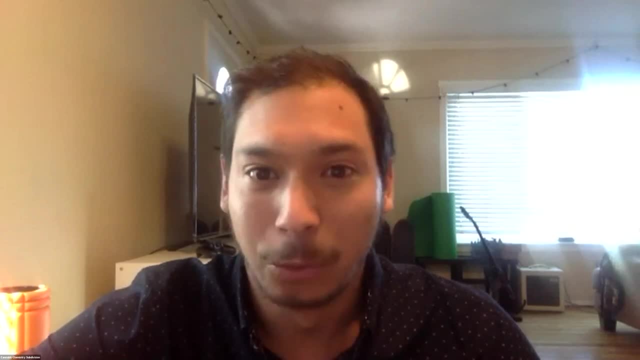 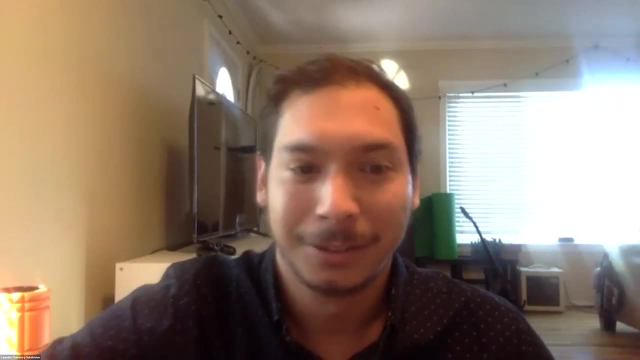 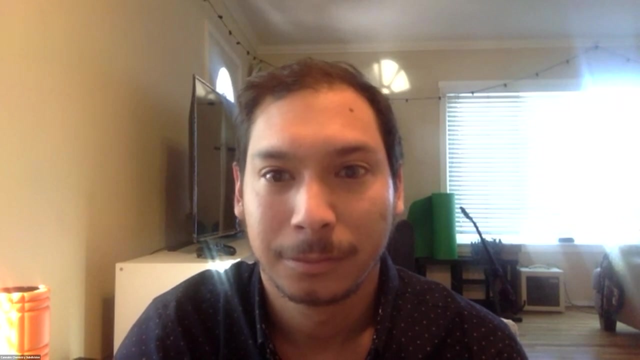 spectroscopy- MPAES. Jenny, we're really pleased to have you today and really looking forward to learning a bit more about your methods. All right, Thank you, Kyle. Okay, so I'm going to share my screen here. We did a test so we know that it works. Okay. presenter mode. 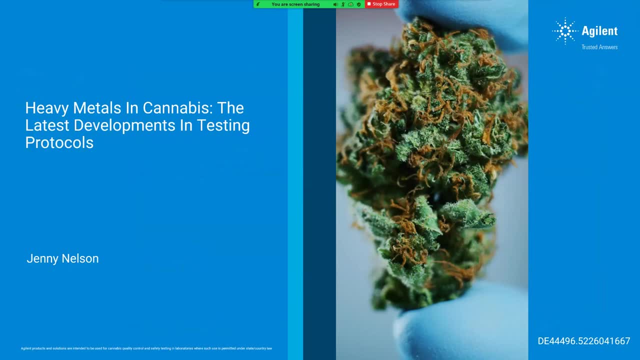 All right, Okay, thanks everybody for joining today. Hopefully there's a mix of metals and non-metals people, but everybody's interested in learning about metals and cannabis, because that's what we're talking about. So today I'm going to talk about heavy metals and cannabis and the 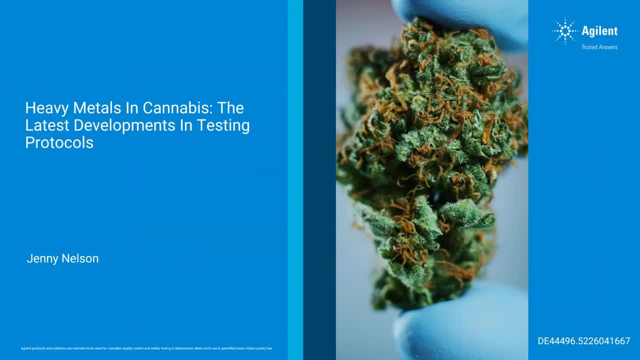 latest developments in testing protocols And I've been very involved with the testing protocols for heavy metals and cannabis for the last few years. I've been working with mostly AOAC and more recently ASTM to develop some of these new testing protocols for heavy metals and cannabis. 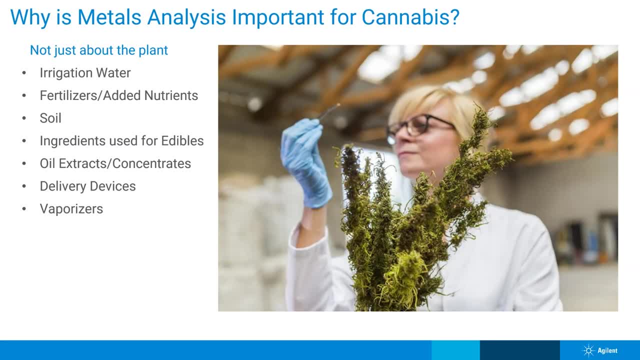 So why is metals analysis important for cannabis? Well, it's not just the plant. actually, Most people think of doing metals testing for the actual cannabis plant, but it's actually more than that, And we get a lot of requests from cannabis customers that they're also interested. 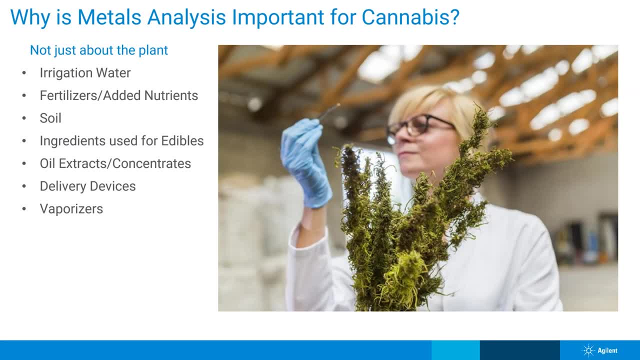 in looking at metals in maybe their irrigation water, the fertilizers and the nutrients that they add to the plants, Also the soil, because obviously these are plants. So cannabis plants can uptake a lot of metals and minerals that are in the soil up into the plant. 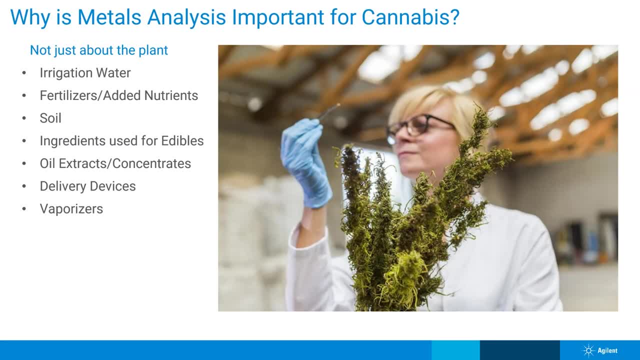 So they want to know that soil before planting cannabis in it. Also, ingredients that are used in some of the edible products: oils, extracts and concentrates. Some of the delivery devices. you might have been hearing a lot recently about things testing and method development around some. 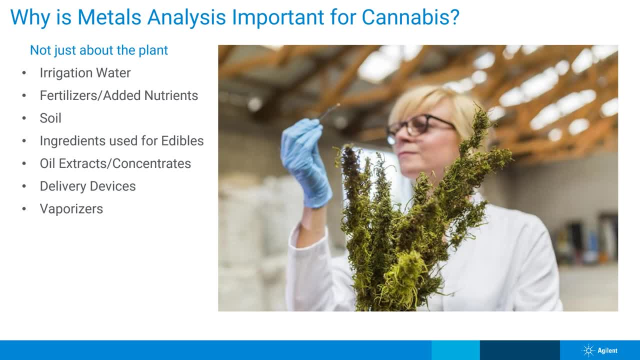 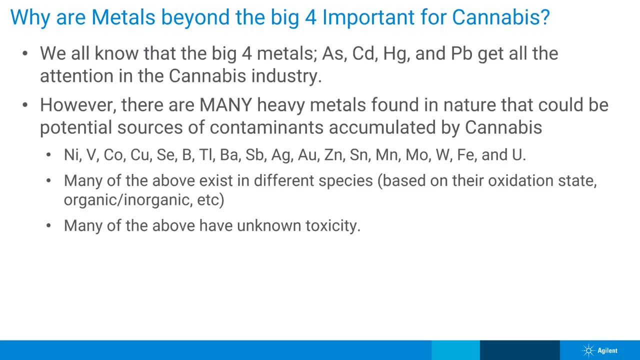 of these devices that people are using these days, And also the cannabis plant, which is a very popular product, And also vaporizers. So you can see there's a long list of things that people are interested in testing metals for. So most people know that in the cannabis industry. 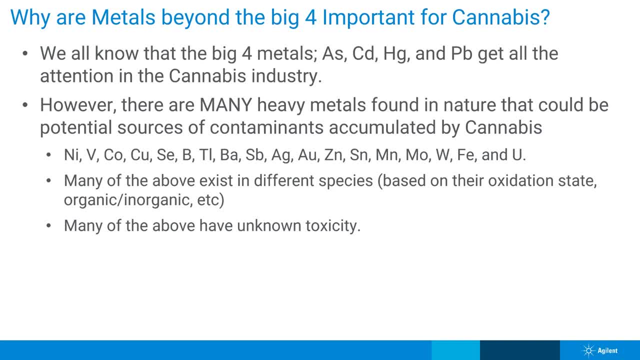 the big four metals- and these are the same big four metals that play a big role in a lot of the food testing as well, And these are commonly known as the big four, the toxic elements, and those are arsenic, cadmium, mercury and lead, And those get most of the attention in the cannabis. 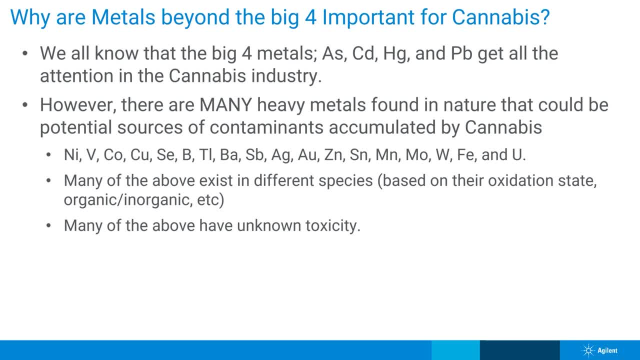 industry, since those are known to be the most toxic, carcinogenic compounds, And so they get a lot of attention. But there are other heavy metals that are found in nature that could also be potential sources of contaminations for cannabis and cannabis-derived products. like some of them, 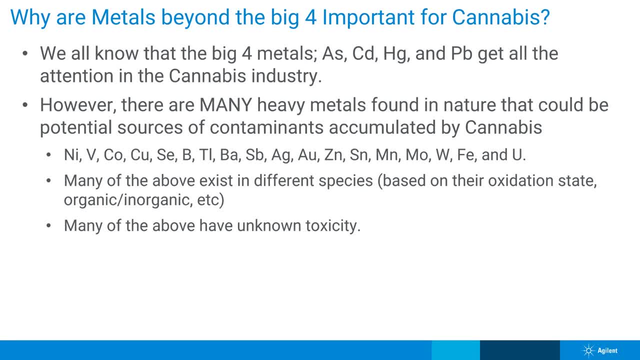 that we talked about earlier, like the edibles, and actually in many of the things that people are consuming these days And some of those metals that are of interest that are beyond the big four are nickel, vanadium, cobalt and zinc, And so they're known to be the most toxic, carcinogenic. 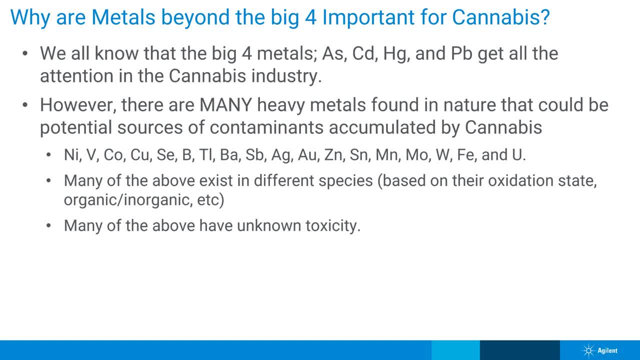 compounds, And so they're known to be the most toxic carcinogenic compounds, And so these are copper, selenium, boron, thallium, barium, antimony, silver, gold, zinc, tin, manganese, moly tungsten, iron and uranium, And those are just some of the ones that we hear from our 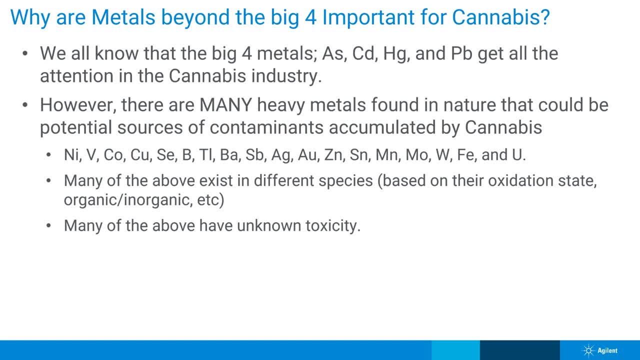 customers that they're interested in testing. However, a lot less work and studies have been done looking at those heavy metals versus the big four, And so there's a lot of things that still need to be studied and we still need to know the toxicity of some of those. 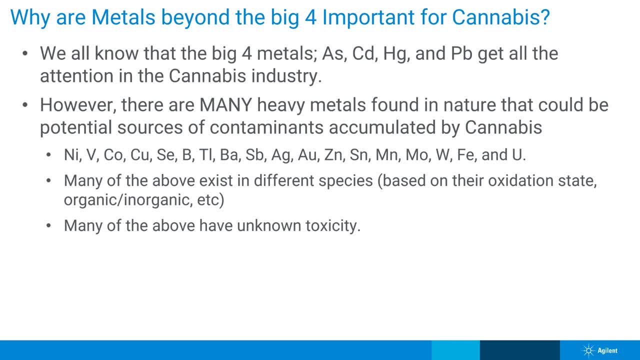 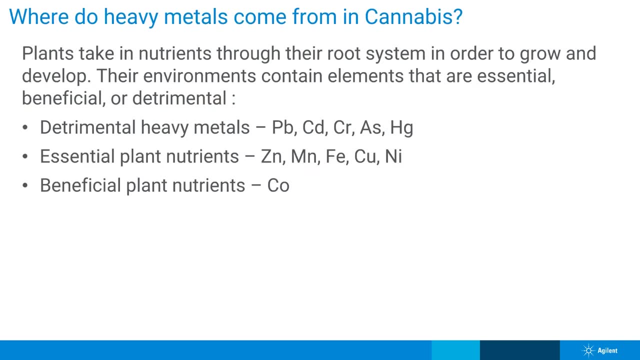 heavy metals and also how they're existing in the plants. So, based on maybe, we want to know what their oxidation state is, or if they're in the organic or inorganic form, and those are just some of the examples. Okay, so plants take up nutrients, which we already briefly talked about. 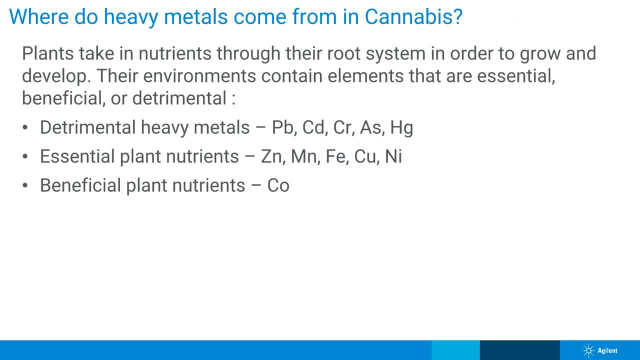 and that they come through the root system in order to grow and develop. And many of these elements can play different roles for the plants. They can be either essential, beneficial or detrimental to the cannabis plant, And some of the detrimental heavy metals are those big four. 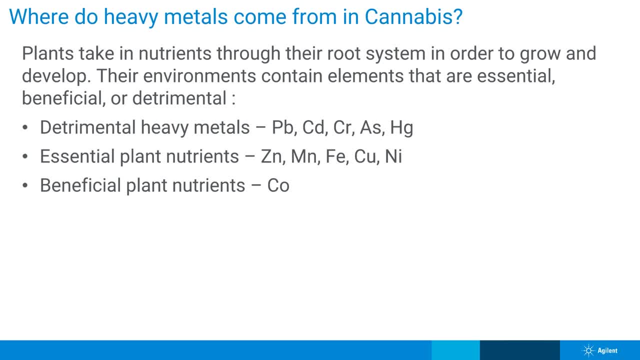 like we just said, like lead, cadmium, arsenic and mercury, but also added to that list is chromium. And then we also have essential plant nutrients and these really help the plants grow, And some of those are zinc, manganese, iron, copper and nickel, And then some that are 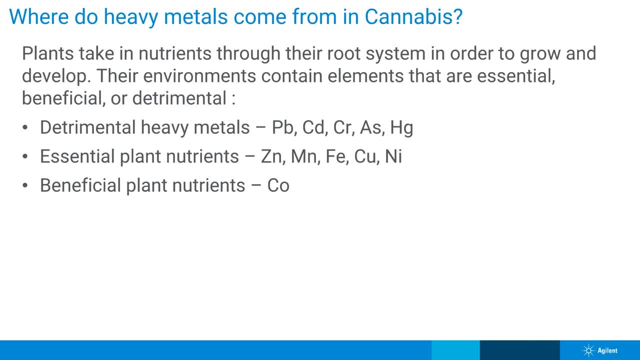 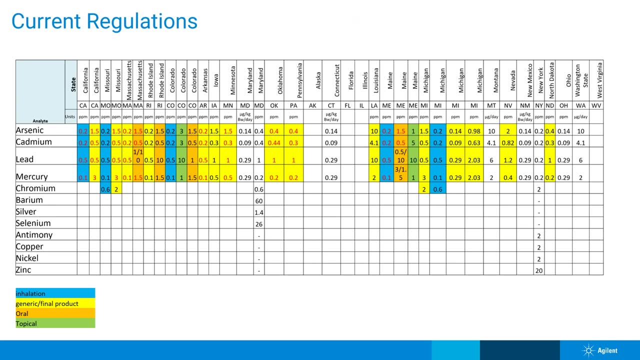 beneficial to plant nutrients would be. one example would be cobalt. Okay, here is a list of, I think, the most up-to-date list we have so far, and these are constantly changing and as states come on board with their new regulations and states that previously had. 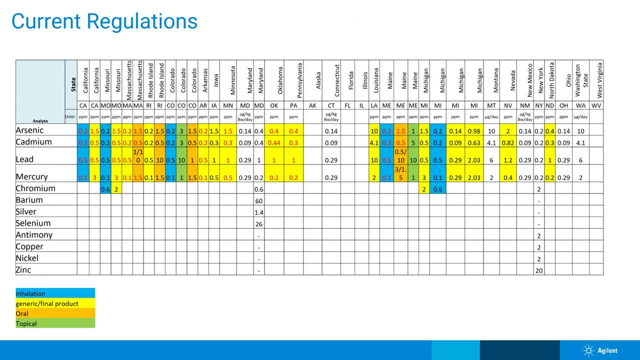 regulations that are updating them and changing them. This is the most current list that we have today, although you know, maybe tomorrow something, some of these numbers will change, But you can see we have quite a few states listed here, So you can see the top of the columns. 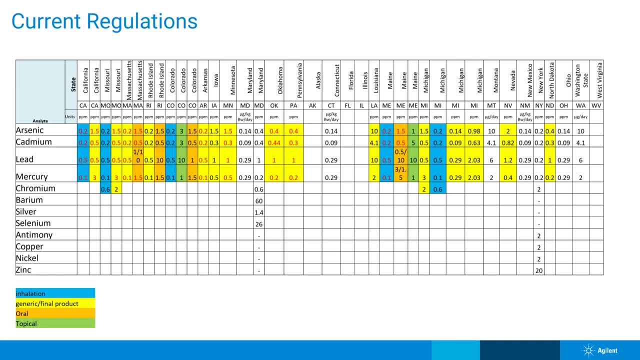 you can see some of the states And then along the side- I'm not sure if you see my cursor or not- let me get my little pointer, laser pointer, So you can see the states up here on the top and then the analyzer, the elements of interest, down the rows right here And you can. 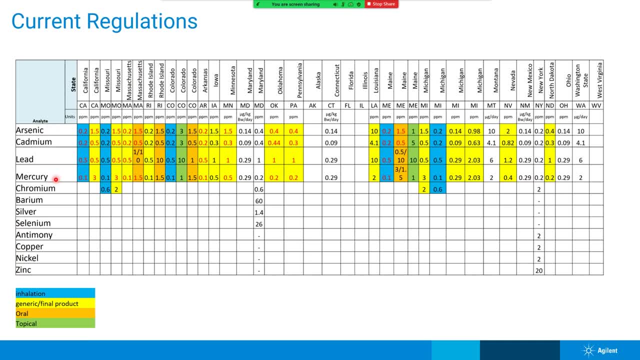 see the big four. So most every single state has that, do have regulations, have regulations for our big four: arsenic, cadmium, lead and mercury. And then we have this like additional, or we'll call it the additional elements right now. So chromium, barium, silver, selenium. 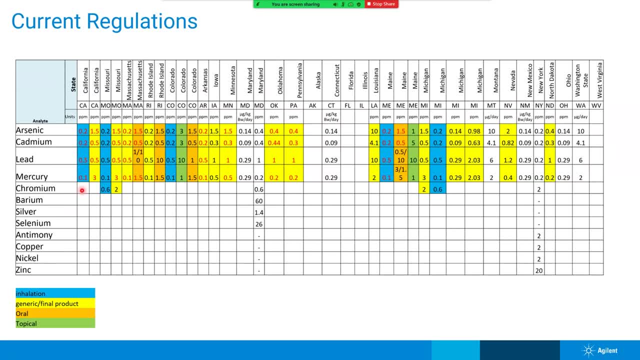 antimony, copper, nickel and zinc. So there's some states that have started to have regulations for these additional elements And you can see right here Maryland did. I think this might not be the most current Maryland ones. I've heard there's been some changes for Maryland, But you 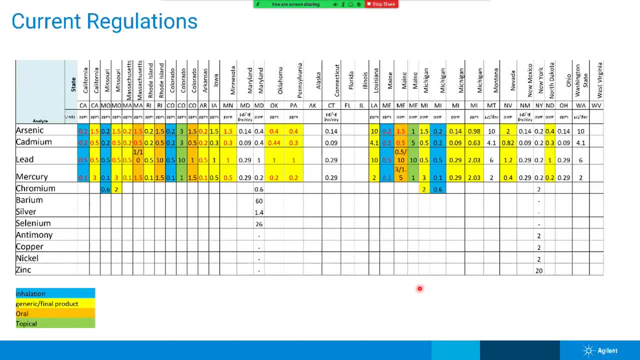 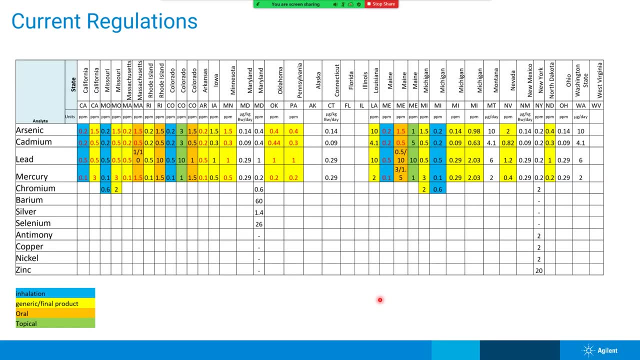 can see for Michigan- they have some listed here- and New York. So again, this list is always changing And it's hard to keep up to date with everyone. since this is state by state, You can also see that some states they change. 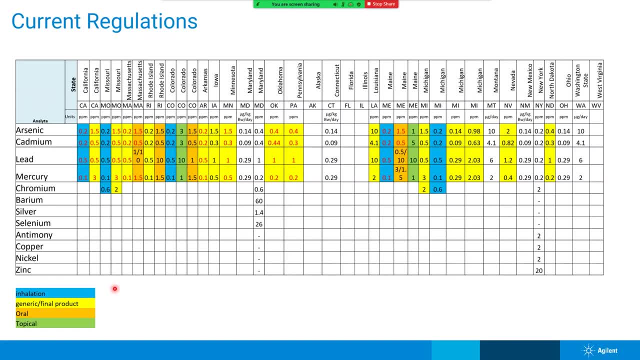 the regulations based on the type of product. So you can see some things are highlighted in blue and that would be for inhaled products, Yellow would be for final products, Orange would be oral and then green would be topical. So it just depends on the product in the state. 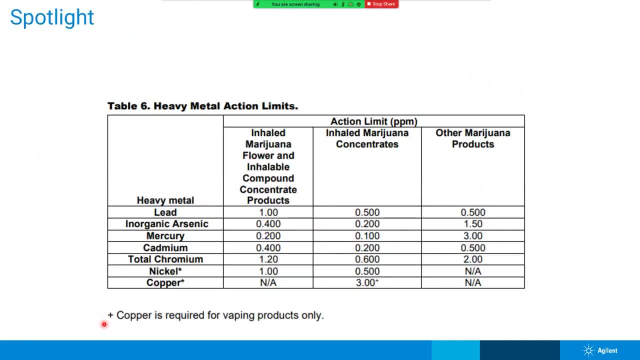 what the regulations are. One state that I did want to point out, that was is Michigan, And this is a newer regulations, I believe, And you can see, on top of the big four elements- so the lead, mercury, cadmium and arsenic- we actually have Michigan calling out inorganic arsenic And 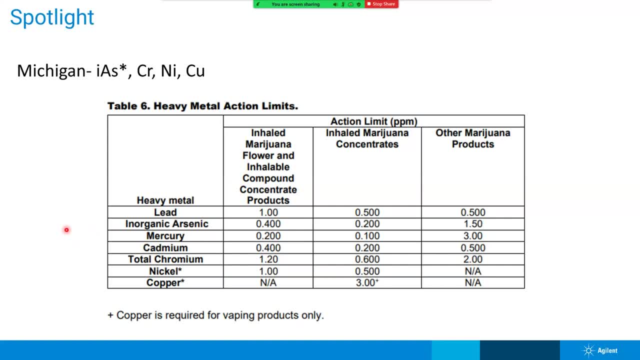 this was actually a surprising thing to me, And that's because inorganic arsenic needs to be tested doing speciation analysis- And I'm not going to talk about speciation analysis, but I've done it for many, many years, And we could have a whole hour talk just on speciation in order to determine. 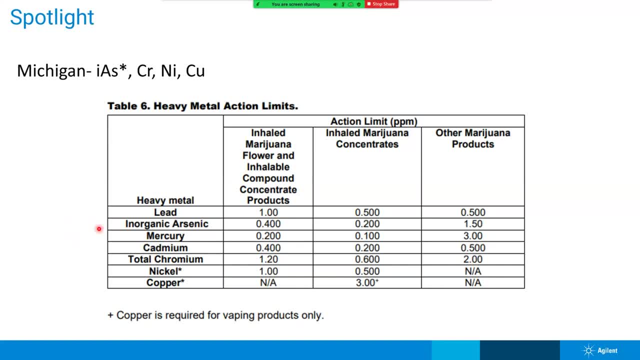 the inorganic arsenic levels, Because most of these methods that people are doing are total methods and we're looking at the total amount of arsenic and not necessarily the inorganic or the organic forms of arsenic. So this was very surprising, And I'm not even sure the Michigan officials that. 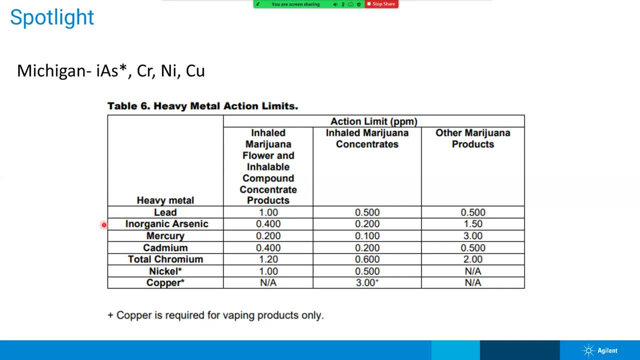 set this and if they know that this would actually be two different methods if you need to determine inorganic arsenic versus just regular arsenic. But it's not surprising, because inorganic arsenic is known to be- it's- the most carcinogenic form. 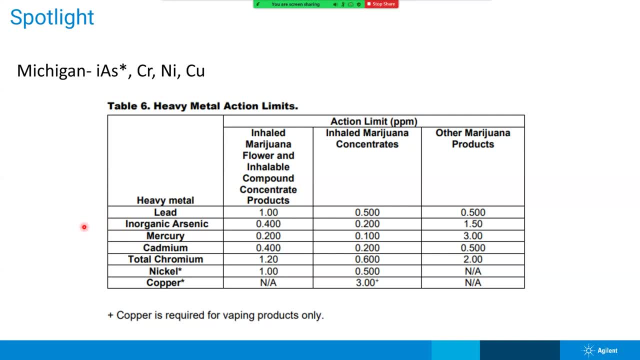 of arsenic and it's the form that's most regulated in the food space. So this would be for like right now: baby food has inorganic arsenic levels that are in Congress right now, And there's different levels of inorganic arsenic for juices and rices and many things. Okay, But 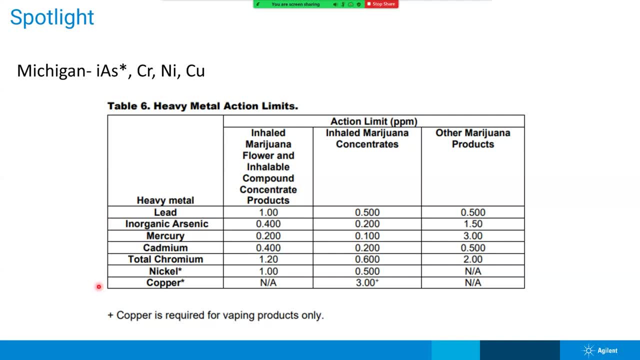 also added to this list that I wanted to point out was the nickel and the copper, And the copper is just required for vaping products. So you can see how it gets quite complicated if you're probably one of these labs that are testing for all these things and all the different levels that are. 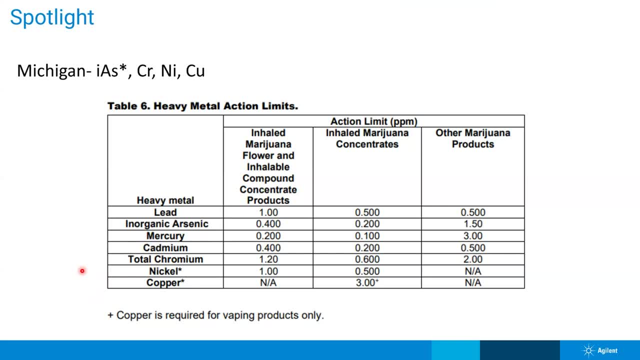 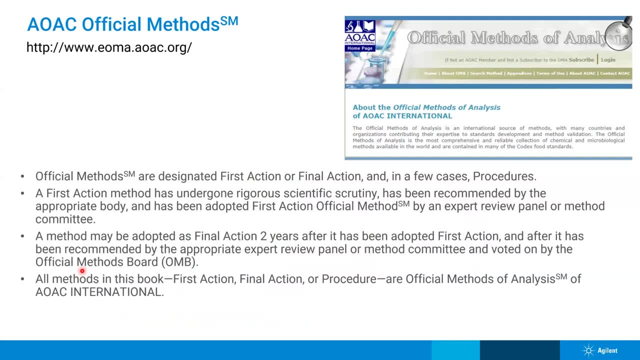 available. depending on the state and depending on what product, it can be quite confusing. Okay, So a few years back, AOAC- which is one of the organizations that I've been working with or volunteering with to work on some method development- they got a cannabis group together. 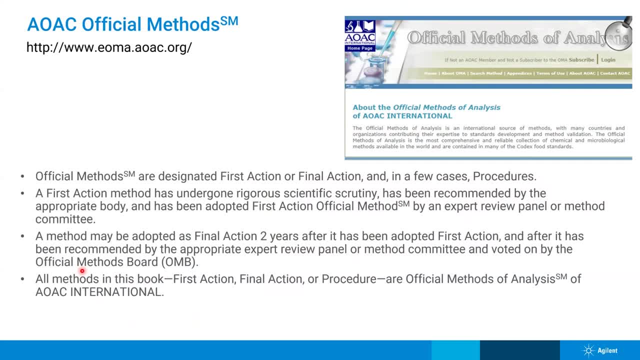 And then I would say over a year ago now, I'm not sure the exact date- they sent out a call for methods, And so this call for methods was for all different cannabis methods, And what it did was it sent out a call for methods for all different cannabis methods And 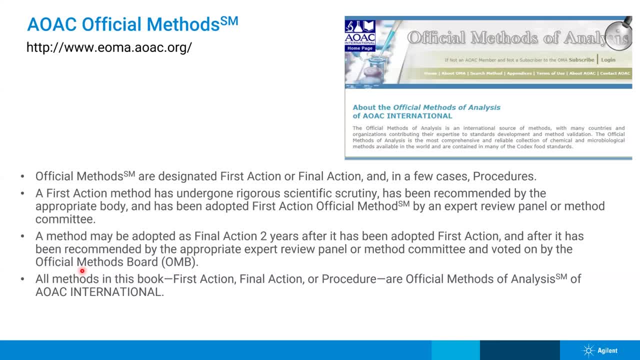 we would look at different methods and we would look at different methods and we would look at all different. One of them was for heavy metals, And so I've been working with AOEC for over a year now to work with them to get a method. 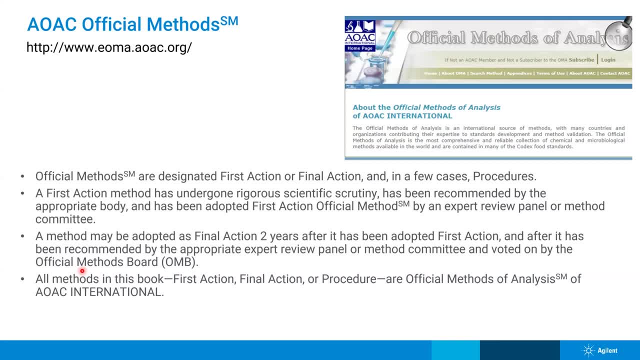 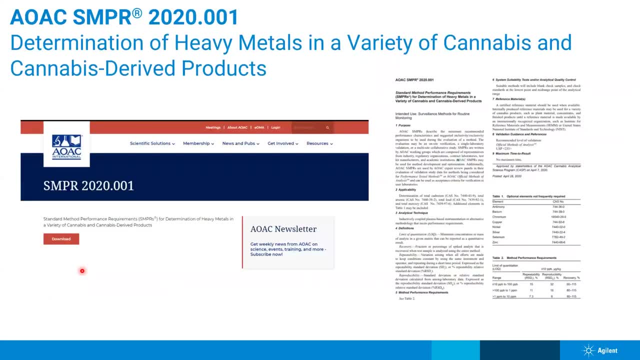 that met their cannabis expert, SMPR. So I'll share with you next what the SMPR is. So this is the SMPR, So this is a standard method performance requirement. So this group at AOEC, which is the cannabis experts, and this is comprised of a whole 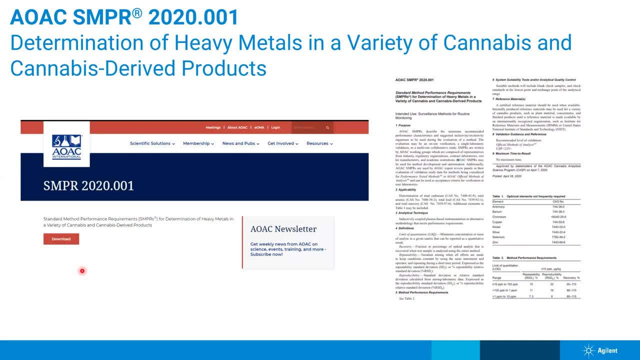 bunch of different people from government to industry, growers- you name it- lab people. This is a large group that came up with this performance requirement. So they set out and they said: we're looking for methods that will measure these heavy metals and the method has to meet these requirements. 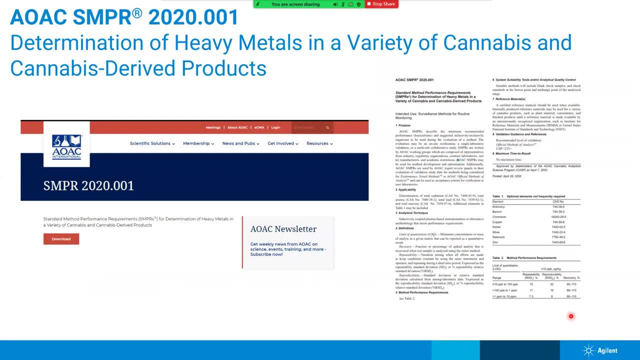 And you can see. I have listed here on the right-hand side of the screen, the performance requirements for this method. So it's saying this method has to measure arsenic, It has to measure cadmium, mercury and lead. so the big four. 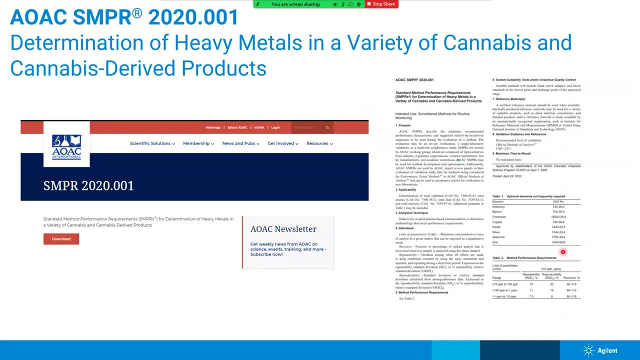 But it also can have these optional elements, which was antimony, barium, chromium, copper, nickel, silver, selenium and zinc, And that is because, at the time that this SMPR was put out, two states which were New. 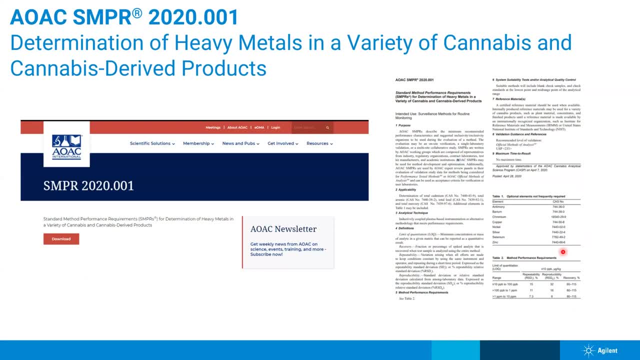 York and Maryland. those were the optional or their additional elements. So that's why that was what it was And you can see down here below the method performance requirements. So for low-level Trace element testing, you can see it's a little bit easier. effects a little bit easier. 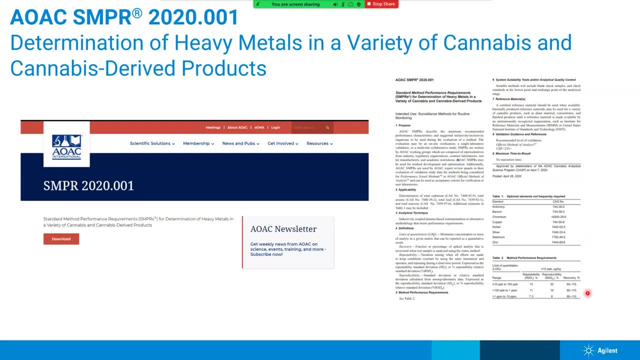 repeatability and reproducibility and recovery, versus when you get to higher concentrations of these toxic elements in the cannabis and cannabis-derived products. OK, so that's the requirements that we were working with for our method, And I had already been working on a metals and cannabis method for many, many years. 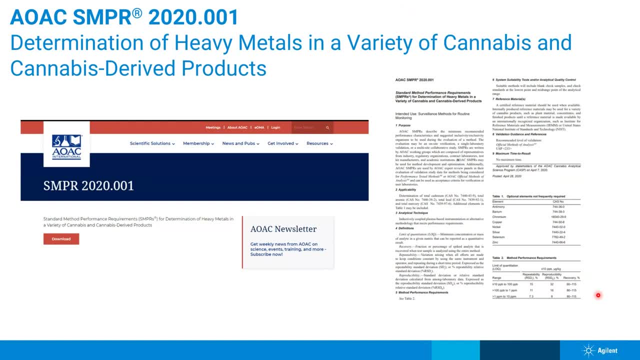 So we just had to tweak our method so it met all these These performance requirements. OK, so we just covered this. I went through that one already, So next we're going to go to the samples. So we need to do this study. 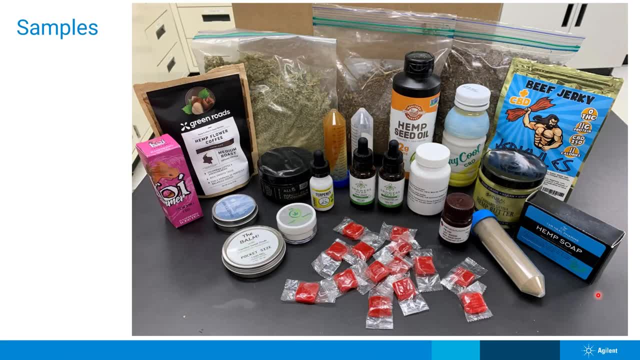 We partnered with a microwave vendor And that's because here at Agilent we do a lot of the testing, So the ICP-MS testing, the metals testing- But we were not experts in sample preparation. So in order to do sample preparation we wanted to work with the experts in that. 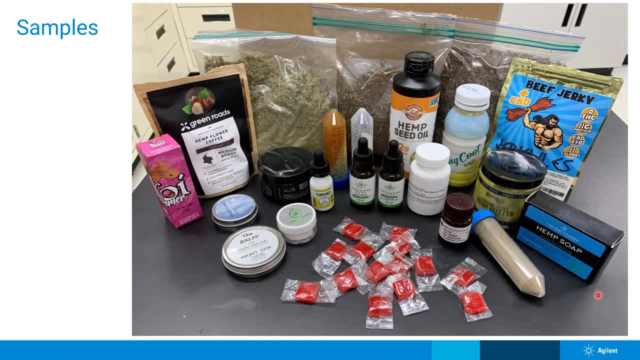 And in our case, we started to work with the EMF And we did a very good job of that And we did a very good job of that. So we did a very good job of that And we did a very good job of that. 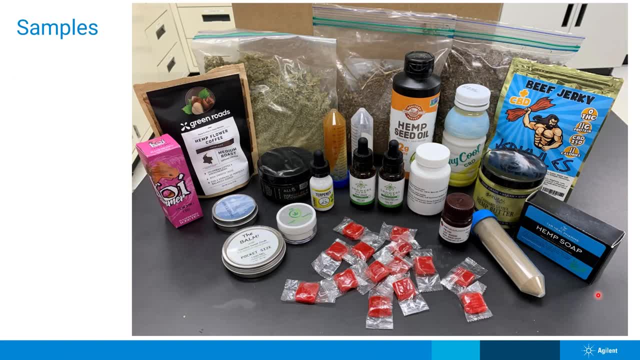 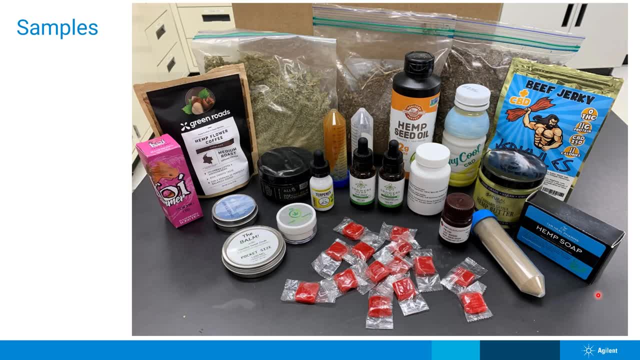 So, in order to do sample preparation, we wanted to work with the experts in that, And in our case, we started to work with CEM, And they're a vendor that makes microwave digestion products, And so what they do is they digest the sample to get it into a liquid form so that we can. 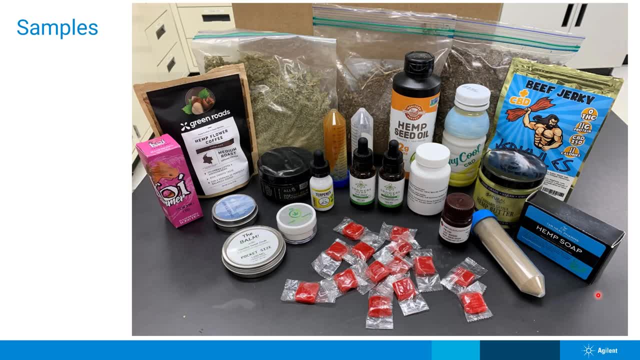 run it on one of our ICP-MS instruments, And you can see here we worked with AOEC And we wanted to get a good group of products that would cover that issue, And so we went ahead and put together an entire range of samples that they were looking. 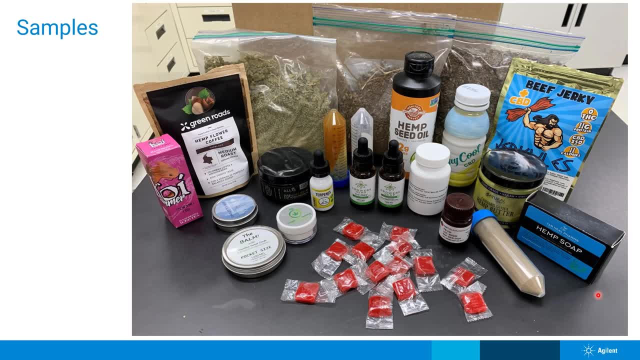 to measure. So again, we're looking at the inhaled, the oral, the topical and the manufactured. So you can see we get a variety of different products here. So you can see, for the oral we looked at different pills or capsules. 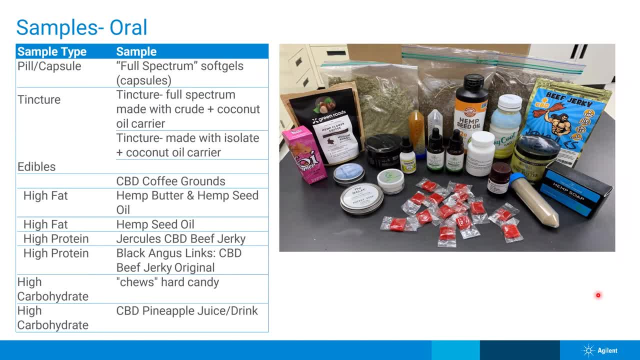 We looked at tinctures And then we looked at edibles, And edibles had a variety of different types of products because we wanted the edibles and we learned this from doing a lot of food testing that you have to have like a set. 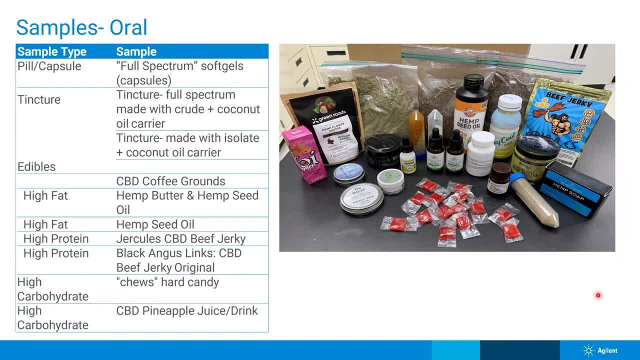 of ways to test the samples, And that's what we did, And that's the role of our lab, And that's what we later did, And that was the goal. Okay, so that's the end of our presentation, like a food or, in this case, edible, that covers the kind of the food triangle, So things that 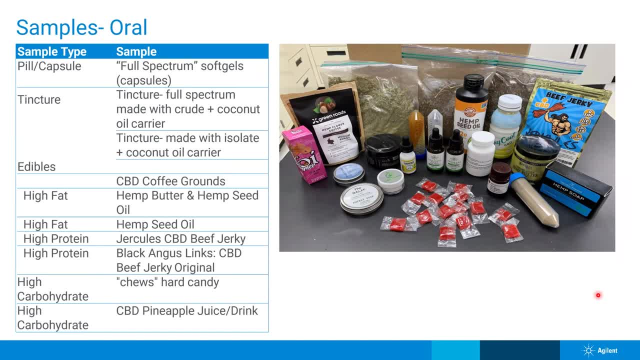 have high fat, high protein, high carbohydrates, so that we could make sure that we could digest everything, since it's kind of a it's tricky to digest things, maybe with high fat versus maybe high carbohydrate, And so CEM folks, they're experts in that and they, they really knew how. 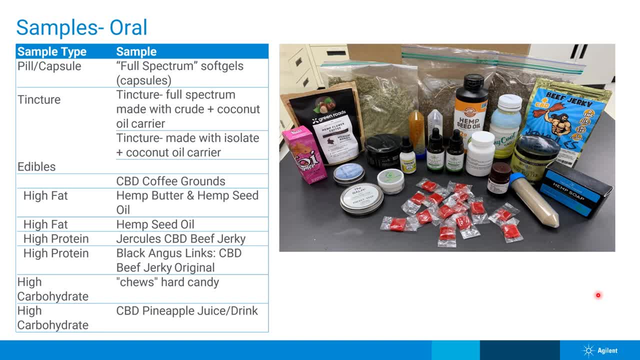 to get everything into solution. And also, I want, I want to point out that we wanted a method that could do all of these different types, all these different matrices, in one method. We didn't want one method that was just for tinctures. We didn't want another method that was for edibles. 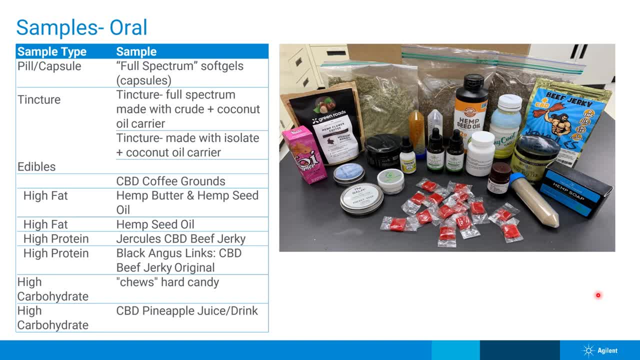 and another one that was just for cannabis flower plants. We wanted a method that could encompass everything and everything could be run in the same method, because we know that in a lot of labs they get, you know, hundreds, if not thousands of samples today, a day, And for them, 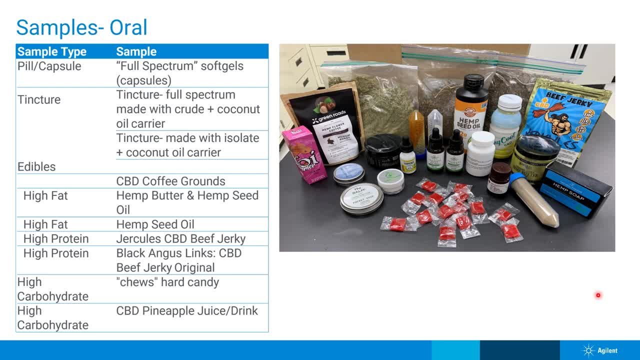 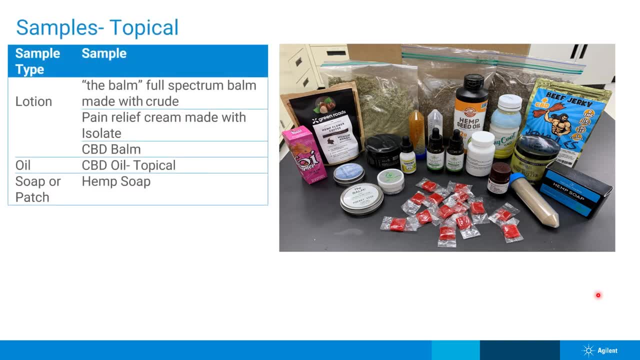 to have you know 10 different methods going on. it's just too confusing And too much extra work, So we wanted to catch all methods. So here are some of the topicals that we looked at. We looked at lotions, oils and soap, And then, for inhaled products, we looked at 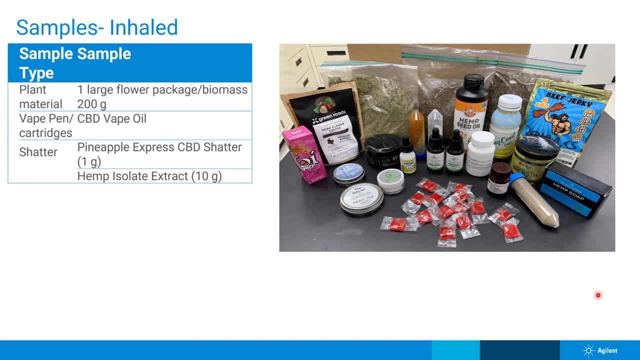 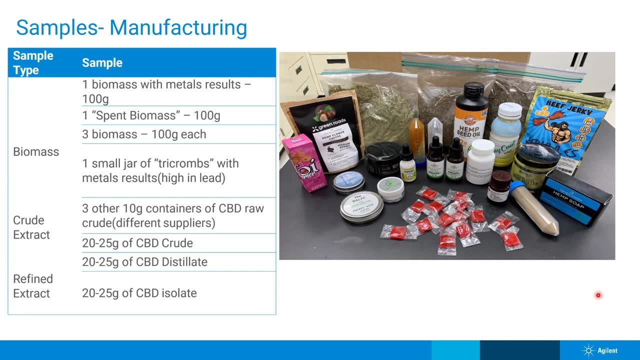 plant material, vape pen cartridges. so the CBD vape oil and then the shatter. So we looked at some CBD shatter And then for the manufacturing products we looked at different biomasses, some crude extract and then some refined extract. So 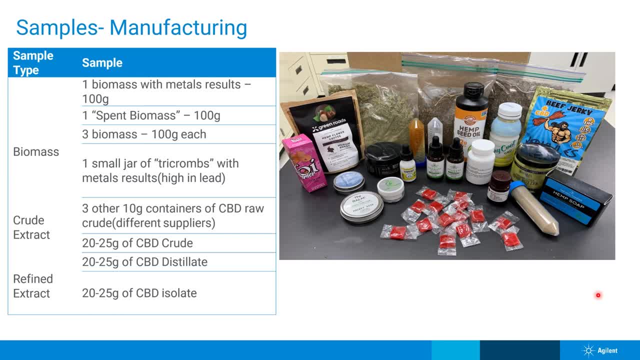 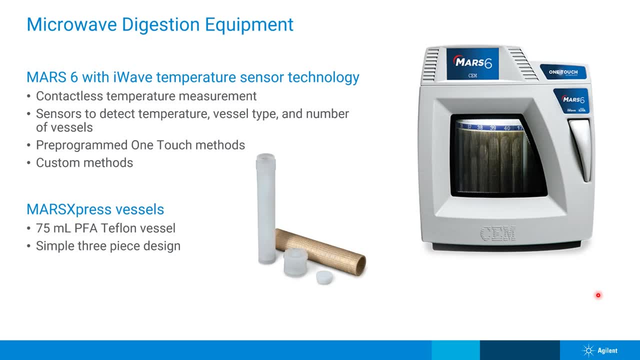 some distillate and some isolate. And then here is a picture of what the microwave instrument is that CEM used to digest all these samples. And since CEM is not on the call with me today, I'm going to play a video from Sam, who is the scientist that I worked with at CEM. 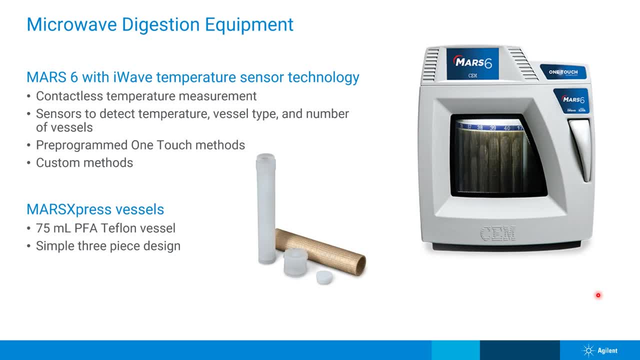 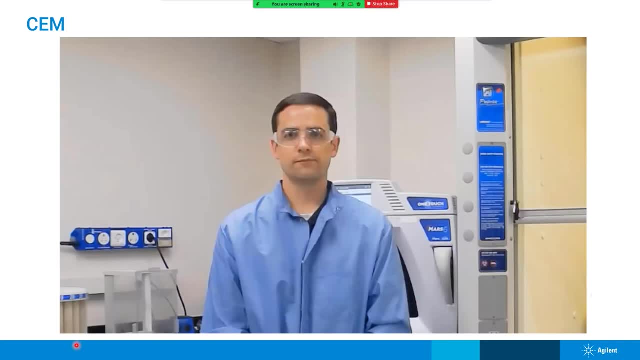 And he is going to show you how he actually digested all of these different types of cannabis products. So Kyle and I tested this already, So let's make sure this works. Hello everyone, and welcome to our lab, As we were talking about, with our AOAC method. 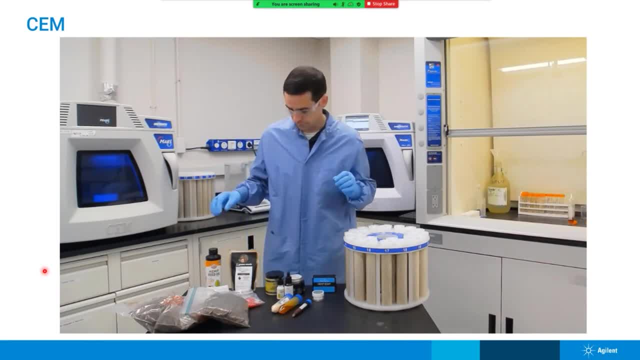 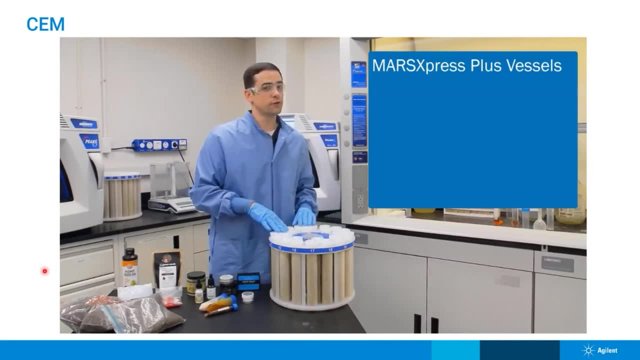 you can digest all of these different sample types using our one AOAC method. All right, We're going to be doing all of this in this Express Plus Mars Express Plus digestion vessel. All right, It's a 24 place vessel using Teflon, 110 mil. 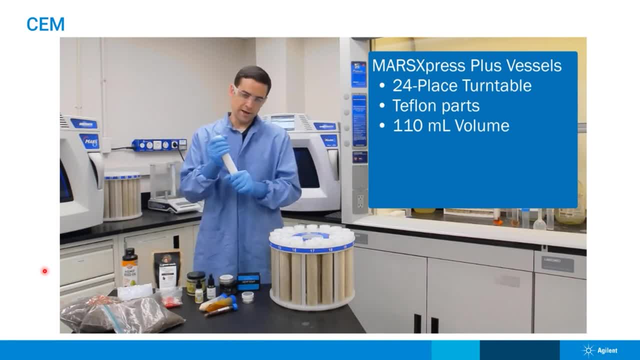 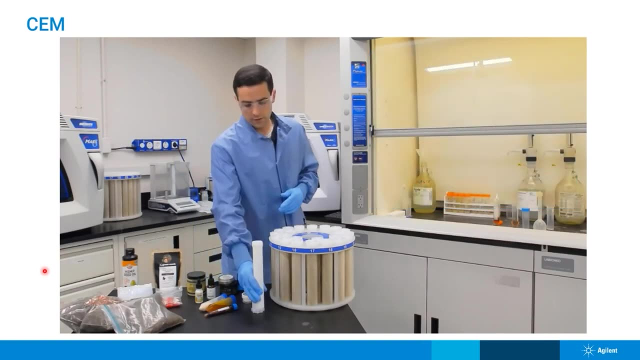 steamer,84 mL normal fuel vessels through a three-piece 날ín assembly with a liner, a plug and a cap. So the liner holds the sample, The plug is for moderating pressure throughout the run and the cap has a hole in it to allow for venting the gasses. 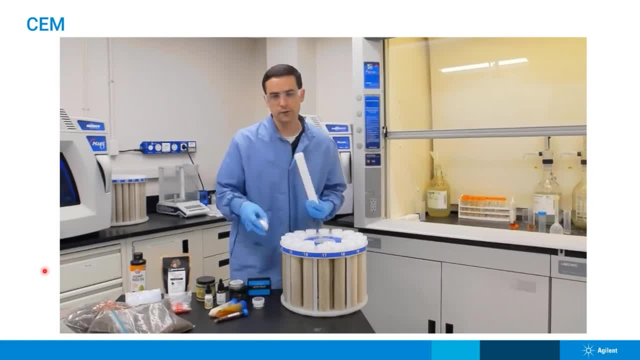 Kyle Ingram 302umbercom. Now let's actually add some sample and show you guys how we do this. So you take your liner Kyle Ingram 302umbercom And you will, typically for plant material, you're going to need a presentation from a leader. so you'll begin to deal with the dry plant bacteria in the PPC7 спасemoney system and we're showing you here what we want you, any specific species that we use where we do need to measure them. And so we're going to dig all of these things out here when we get toок titles from a Columbus site. So you do this. 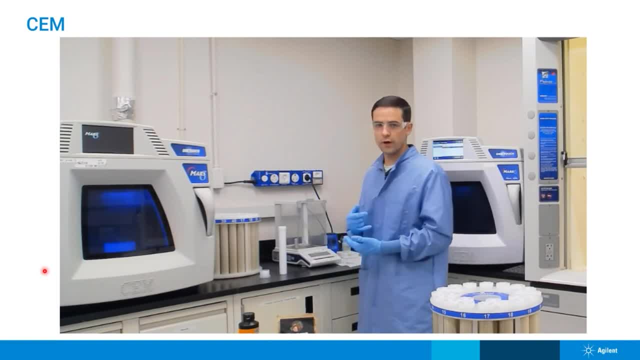 plant material. we would usually use whey paper, whey boats. You want to make sure that you know if you're using these types of things. you want to make sure you're not running into static issues, So we may sometimes put our vessels in. 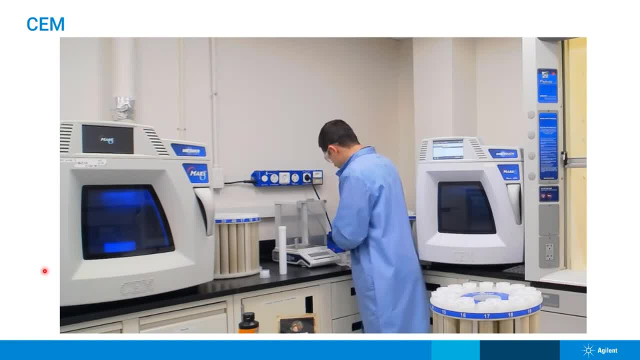 front of an anti-static ionizer like this. That really helps to stop your samples from sticking to the sides of the vessels or sticking to the whey paper itself. right, A good technique for whey paper is to fold it in half It. 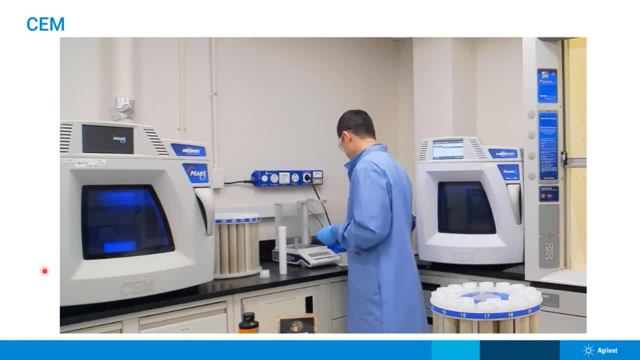 makes it easier to dispense it into your vessels. when the time comes right- And there are a few other techniques that we like to use for you know some of the harder samples to put into your vessels, like the creams or the butters, We typically might use a plastic spatula like this. If you use any type of 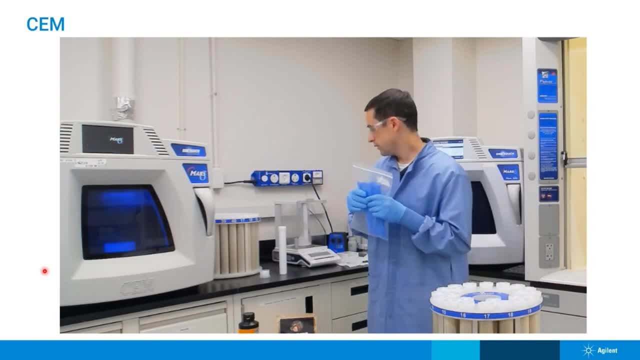 plastic scrupules or, you know, dispense wire. you want to make sure that you clean it beforehand. using glue bags For liquid samples. we like to use these pipe transfer pipettes And again, you want to make sure you clean these beforehand using dilute acid. so 10%. 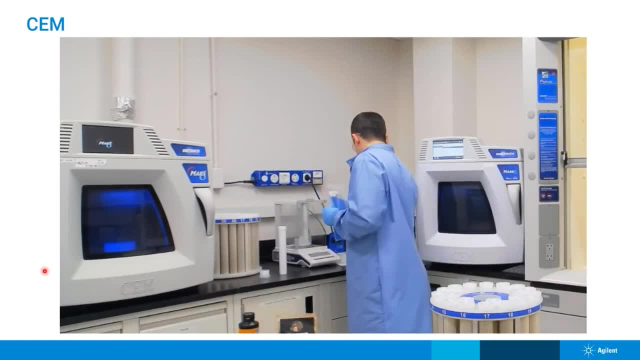 nitro or gray, All right, and make sure when you're adding these samples you get the sample to the very bottom of the vessel. That is very important. You want to make sure that your sample is completely submerged in acid right Some? 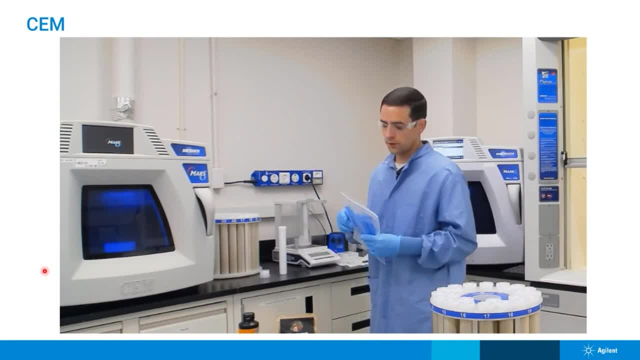 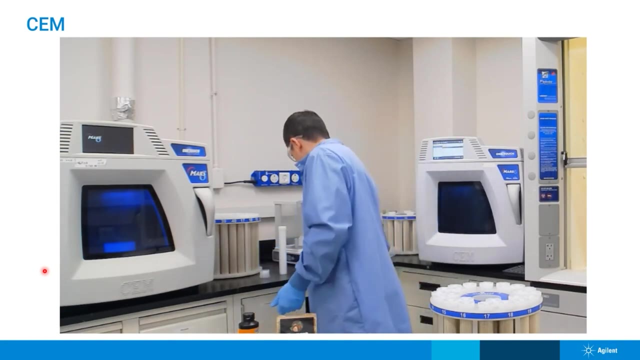 of the concentrates and oils like to stick to the sides. if you want to use these tools to make sure you get it to the bottom, All right, I've got some plant material conveniently already weighed out for me This. well, first let me show you The plant material if it comes in my bag. it 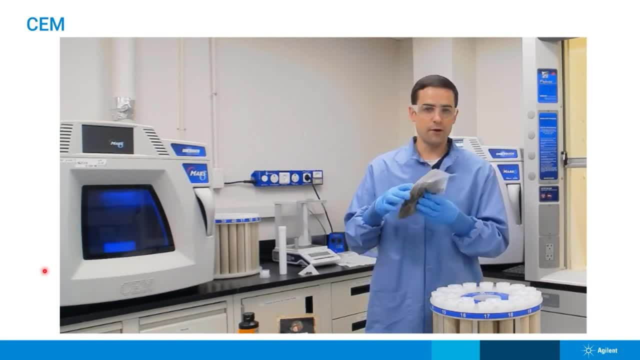 may not be very homogenous. right, You want to mix this bag up? Tumble it a few times, shake it up a little bit, make sure that everything gets nice and homogenous in there, Otherwise your stems might sit on the top of everything and the shaky 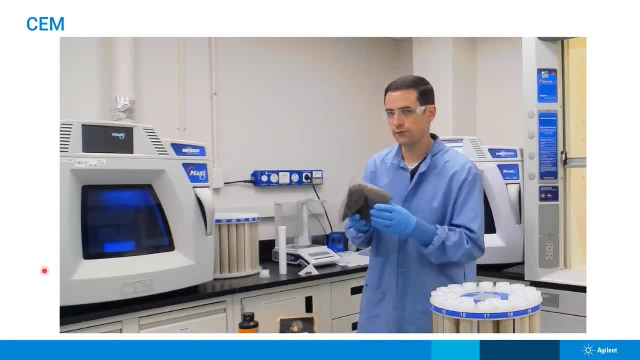 stuff will go to the bottom. You want to make sure you tumble it a few times and get it nice and homogenous before you sample. And when you do sample it don't just take all from one spot. Make sure you take a little bit from here, from. 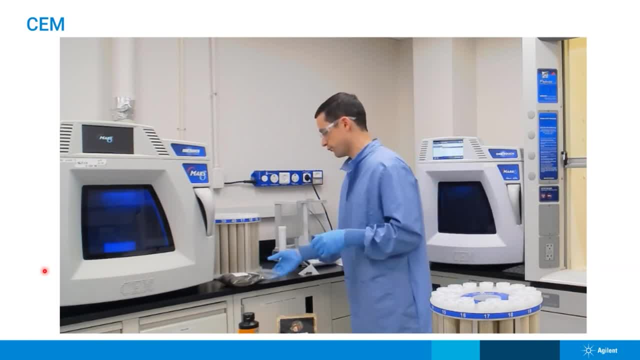 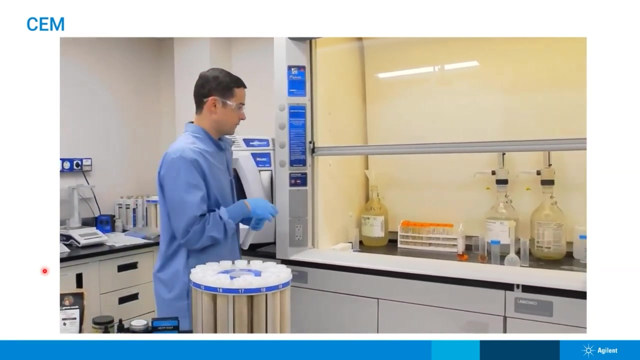 there and get a little bit of everything so that you get a nice representative sample. All right, so you take our pre-weighed out sample and add it to the bottom of the vessel. All right, We're going to take the surface of the hood and add acid. 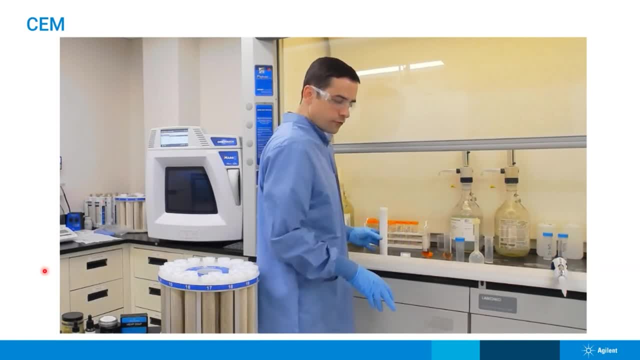 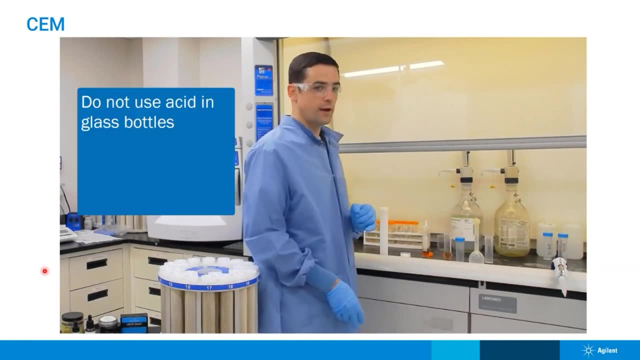 So for our method we call for nine mils of nitric and one mil of HCL. You can see here we have acid in glass bottles. We do not want to use acid in glass bottles. Glass is inherently dirty and it will contaminate your samples. 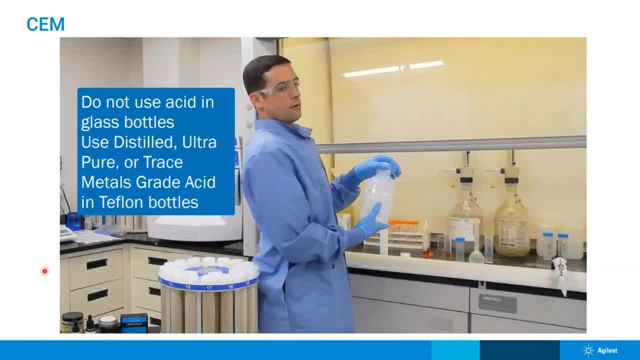 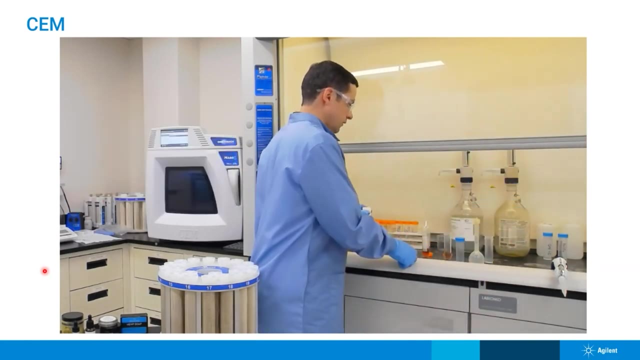 So we tend to use either our own distilled acid that comes in Teflon bottles, or you can order your own ultra-pure teflon. You know reagent grade or trace metal grade acids from a few different sources. All right, so for adding the acid we tend to use micro-pipettes, just because we know. 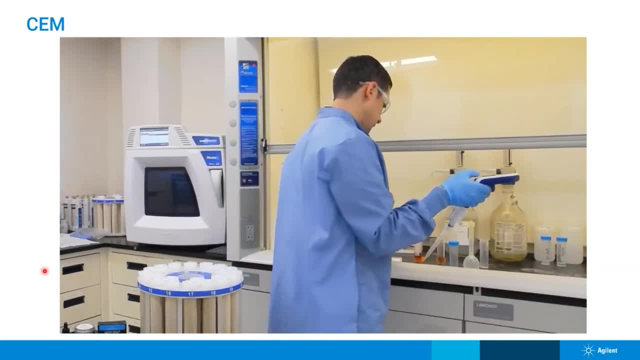 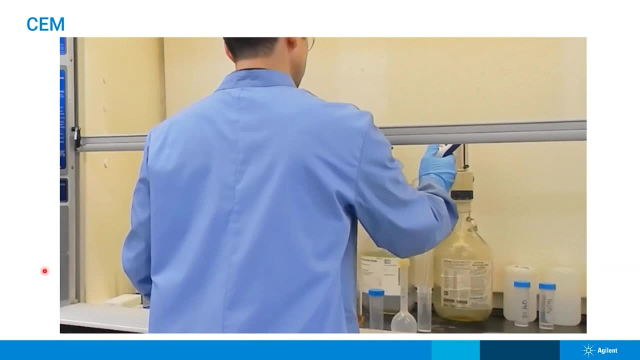 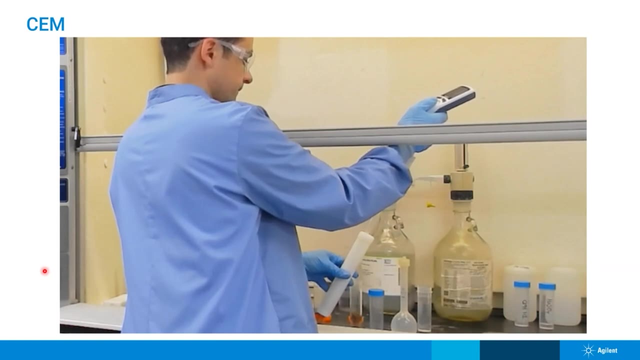 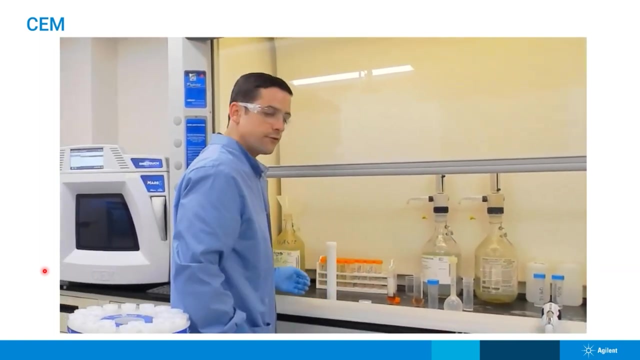 the tips are clean and we know they're very adding. Let me go ahead and add some acid. All right now. once we've added our acid, we'll let it sit and pre-digest for up to 15, maybe even 30 minutes, depending on how reactive your sample is. 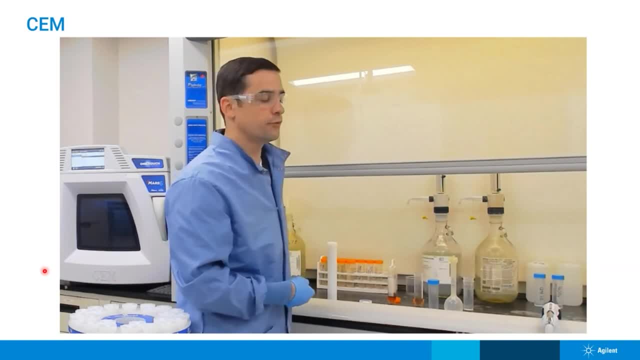 If it's reacting at room temperature, it's a good idea to just go ahead and let it pre-digest. If it's not, then you can just go ahead and fill it up and go. But for most of these cannabis and cannabis throughout products, they're going to react. 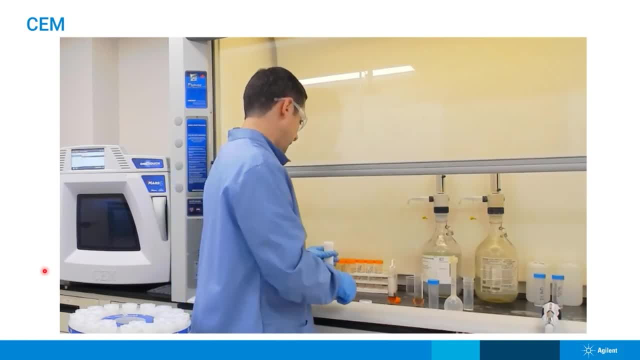 So just let them sit for at least 15 minutes, All right. One thing you'll notice here is that we're going to add acid, All right. So what I'm going to do is actually I have some cannabis plant material already added to this tube with acid in here. 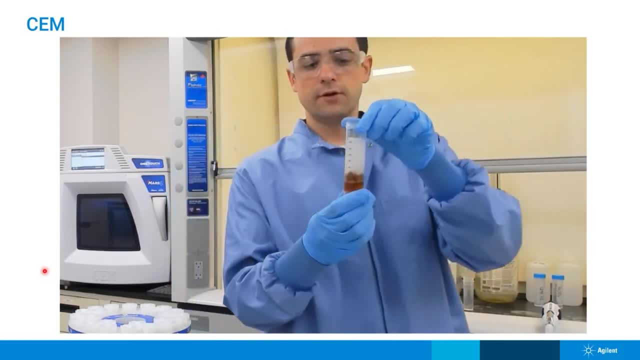 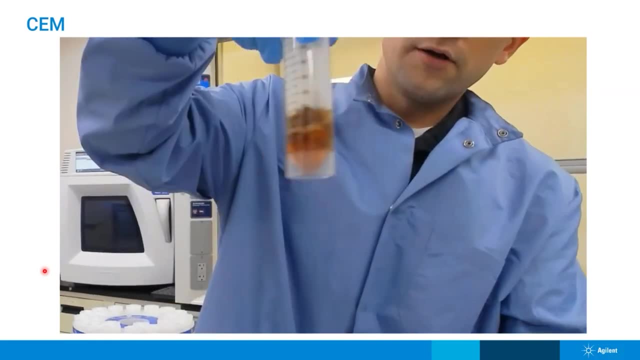 This is 10 mils of acid. You can see, actually, that the plant material is creeping up out of the acid, right? That's not good. You want to make sure that it's submerged, So might swirl it around a little bit just to get it all mixed together so that it runs. 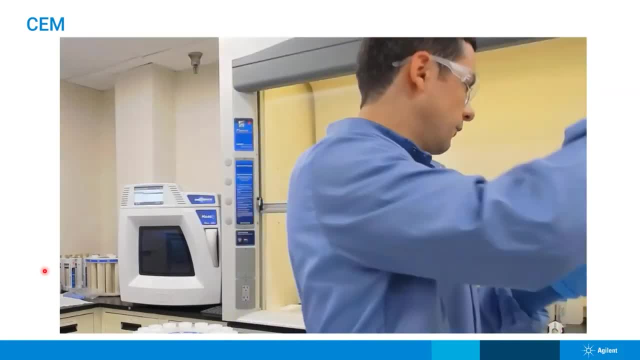 well, You see, it's nice and submerged, All right. What we do not want is to use too little acid, Because then it will all be spent during the reaction. You can see here, this is only three mils of acid. 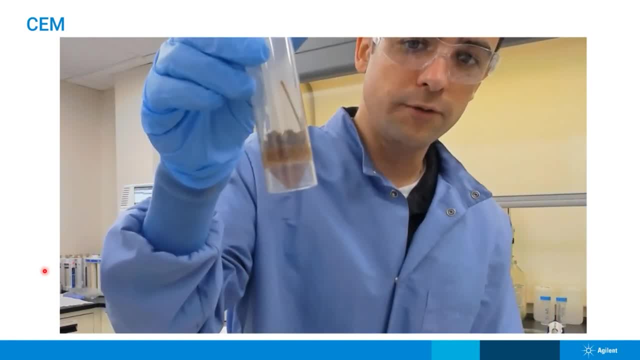 It's not going to completely submerge in three mils And you're going to run into problems And it's just not going to completely digest. So to get around that, we recommend using at least five mils of acid. We would prefer that you would use 10.. 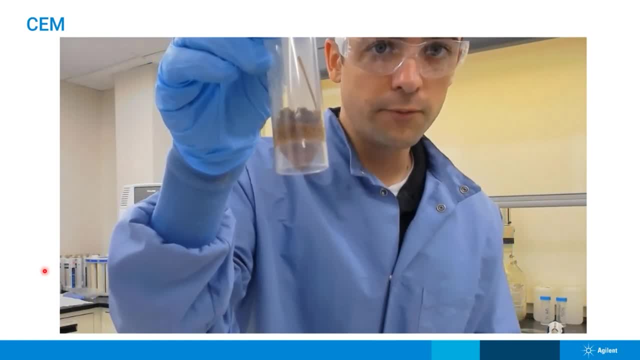 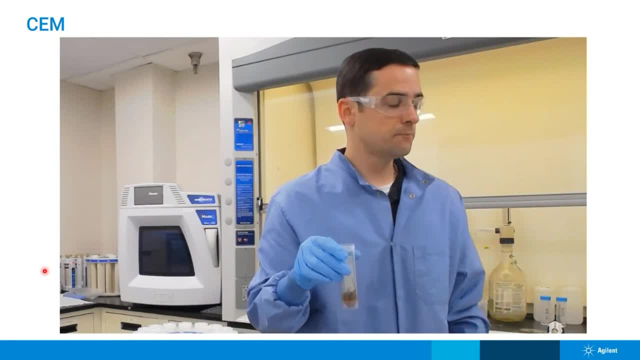 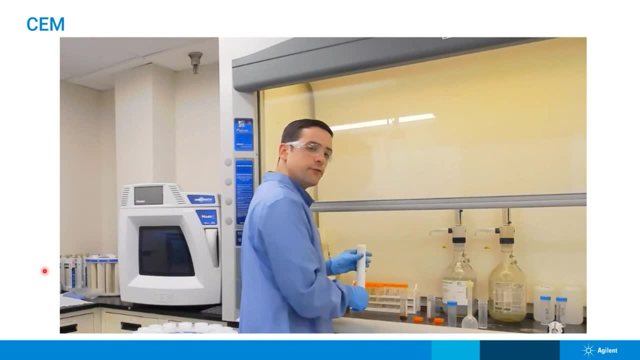 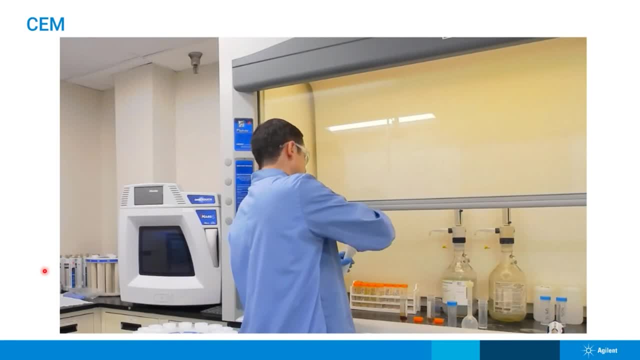 And then pour down our cap. If you gave this to five different lab workers, they would all tore it down, hand torque it down at five different pressures. So what we want to do is use our hand torquing device so that every vessel gets the same. 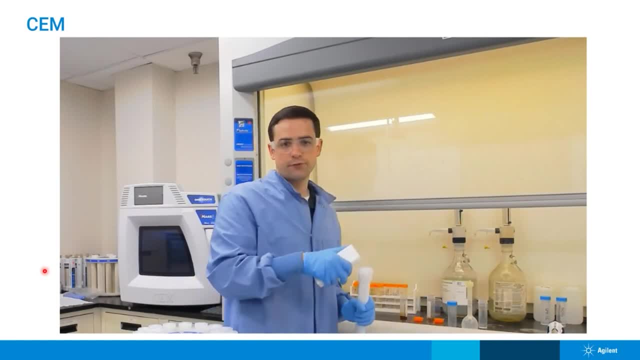 amount of torque, And what that will do is prevent certain vessels from taking off and overreacting while they're. It'll make sure everything is nice and flat and reacts well together, Alright. so now that we've got our vessel torqued, let's go ahead and put it into the 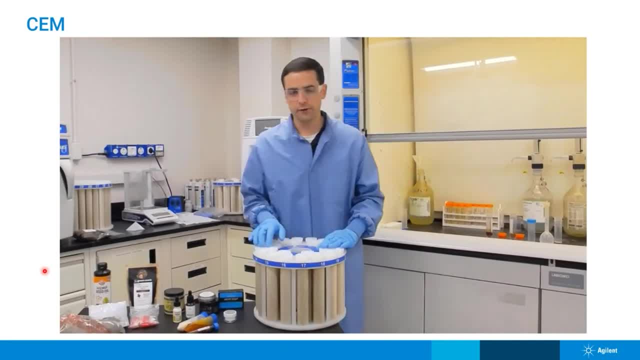 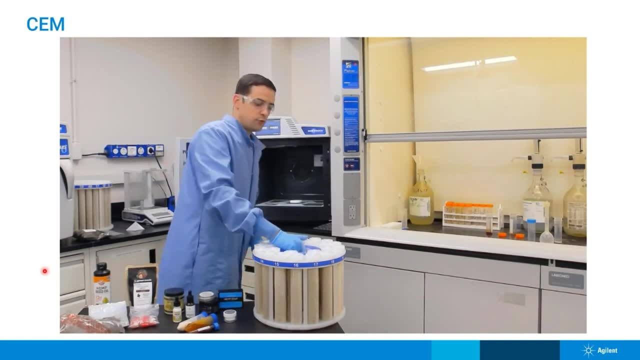 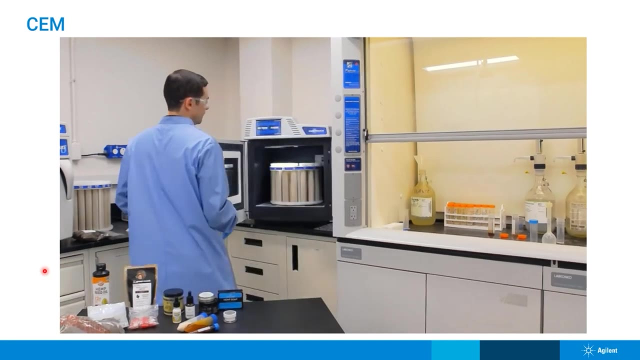 turntable, Make sure it's nice and flush, and then we'll take it over to the microwave. Alright, so we'll take our turntable, put it in the microwave, Shut the door. Then you have two different method directories to pick from. 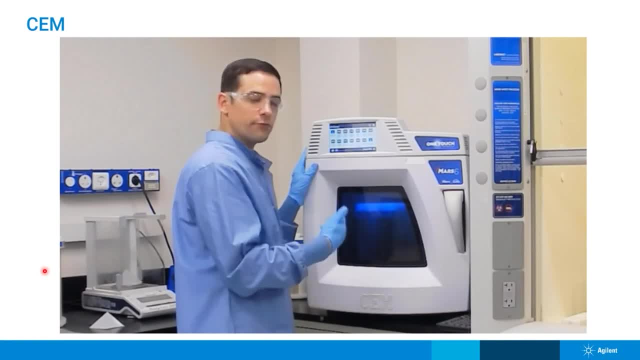 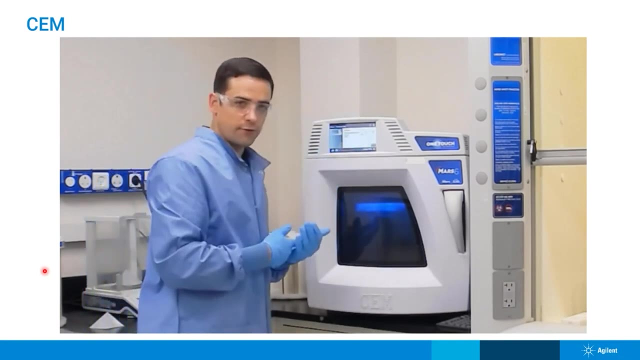 We're going to pick the one-touch directory That comes with all of CEM's pre-programmed methods and you'll find the cannabis one-touch method near the top in the seats. obviously, Press that method and that's it. You hit start and the unit will determine how many vessels you've got in there. what? 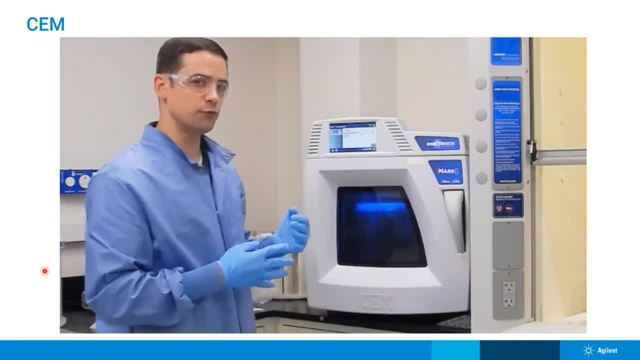 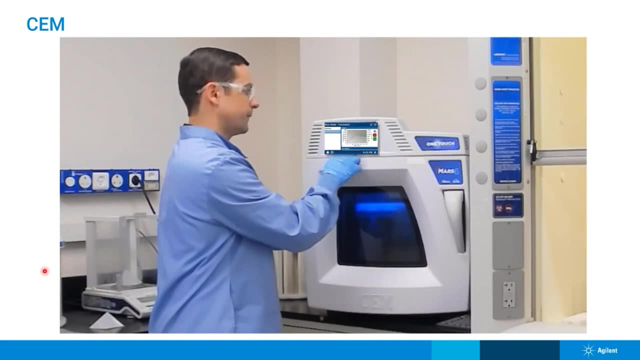 kind of vessels you're using and how much power to apply so that you get there safely, Right? So let's go ahead and look at the run history of our vessel. So the previous run I run you can see here the power starts off low, as does the temperature. 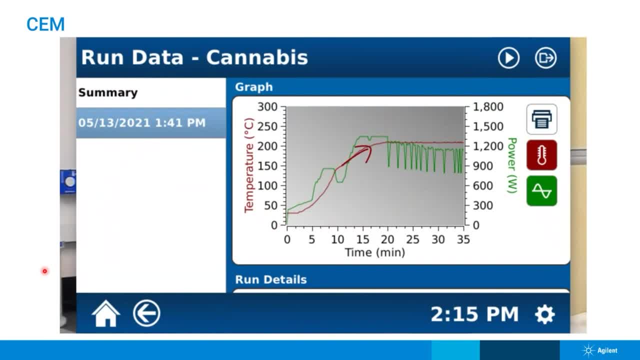 which you would expect, and it slowly ramps it up to temperature. We call that ramp to temperature. It's a very safe way to get our temples all to temperature. you know everything relatively at the same temperature and same pressure, safely. So once we get to the end of the ramp, we're at 210 degrees and you'll notice that the 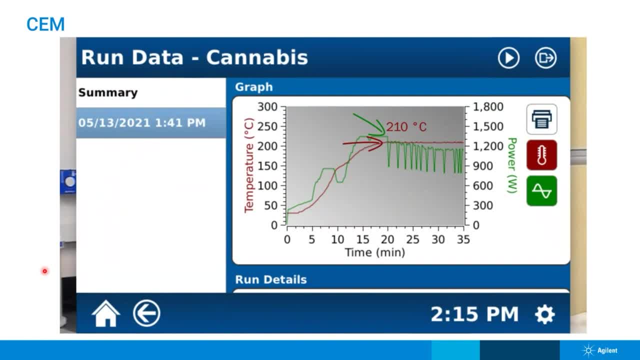 green line, the power, there is modulating to make sure that the red line, the power, or sorry, the temperature, stays steady. Right, You want to hold it at 210 for 15 minutes. After that the samples are digested. 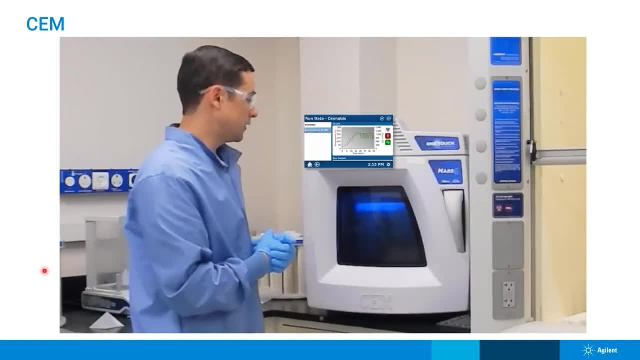 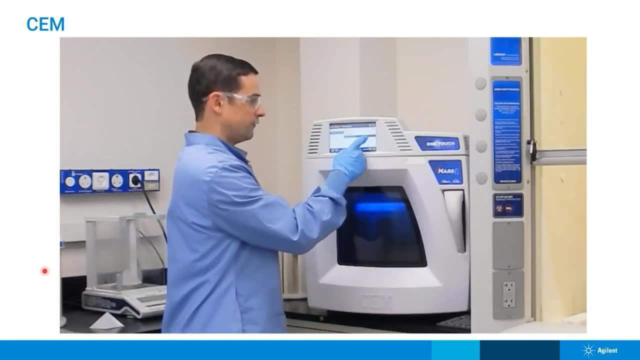 They'll go into a 15-minute cool-down and after the 15 minutes is up, you're able to pull them out and take a look at your digestions. Here I'll show you some of the details of our run previously. 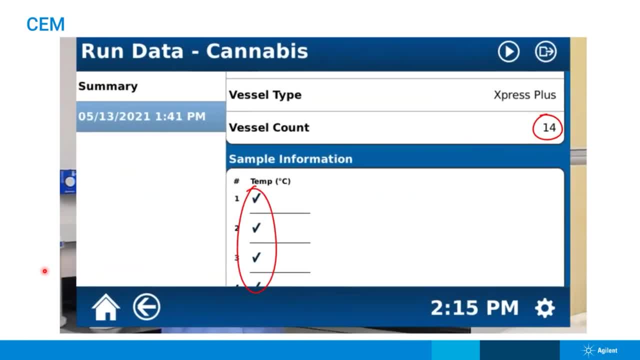 We ran 14 vessels and you can see here the check marks. That just shows that your sample made at the temperature. If you see any X's there, it'll also give you the temperature that that vessel reached and that way you know, oh, my temperature might have dropped. 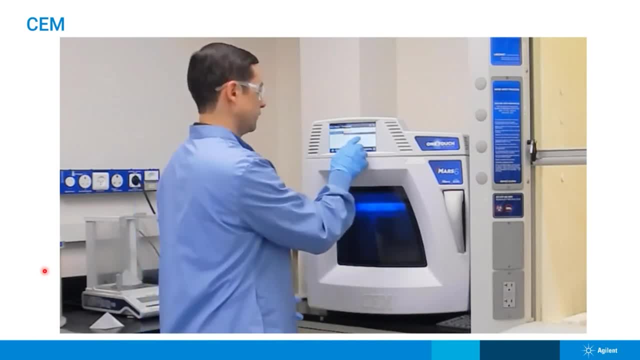 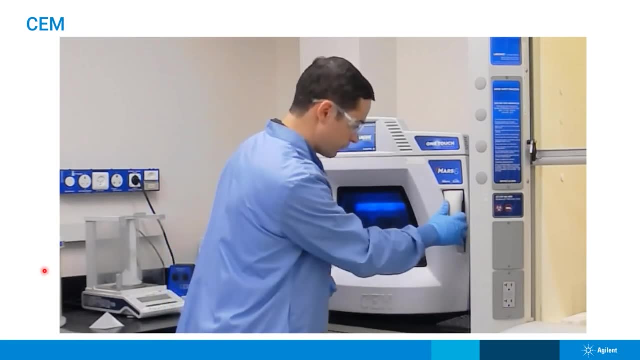 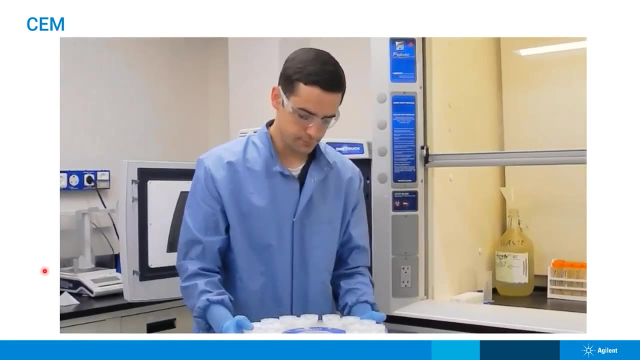 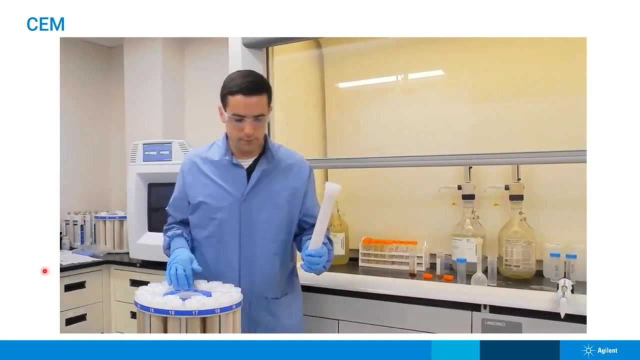 My sample did not make it to temperature. That's why it did not digest. Really helpful tool, All right. So now that our samples are digested, let's pull them out of the microwave and take a look. All right, Now that the reaction has subsided, there is still pressure in these vessels, right? 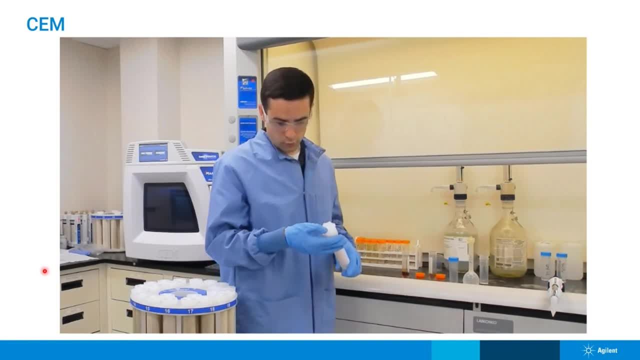 We want to make sure we're safe when we open them Again. there is a hole in the cap to allow fumes to vent out. You want to point that away from you and vent in a pew hood right Like this. You can see the gases coming out of there. 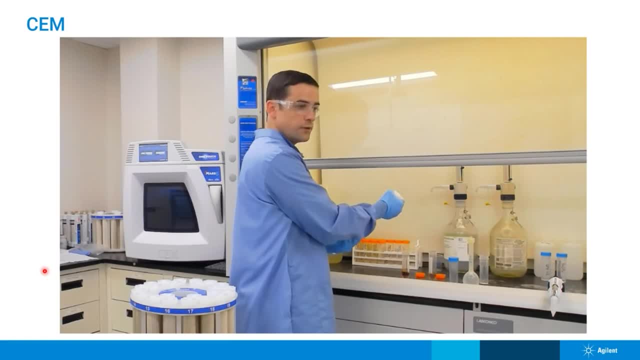 That's what you should expect. There will pretty much always be some type of pressure built up there in the reaction. It's usually carbon dioxide and NOx gases that are formed. All right, Now that we've opened it up, we want to dilute this up. 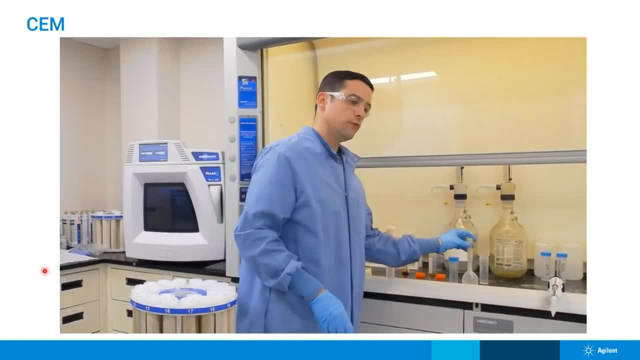 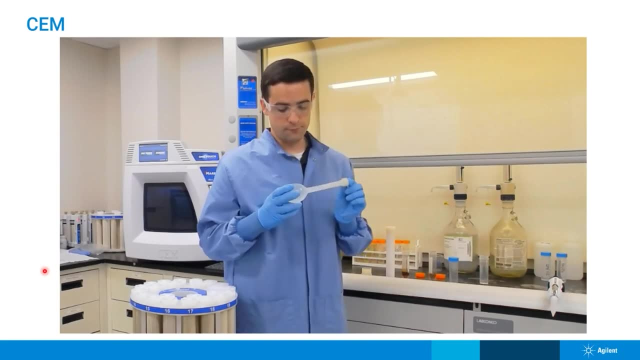 And the way you dilute it up matters. You don't want to use any type of glass, So the two different ways you can dilute it up are volumetrically and gravimetrically. If you're using volumetrics, you want to make sure you use Teflon volumetrics that are pretty. 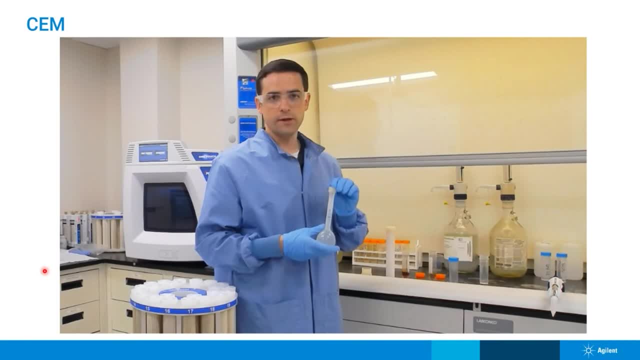 clean. You know, rinse them over a week in dilute acid before you use them. Don't just reuse and reuse and reuse, because you'll get contamination from your samples. All right, Dilute to the line. This is a Class A volumetric. 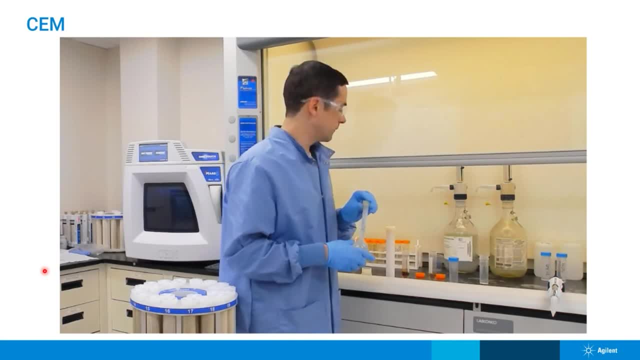 You want to make sure you use Type 1 ASTM water, All right. Another way to dilute is gravimetrically, and this is what we use in our method. It tends to be more accurate. That's why we use it. 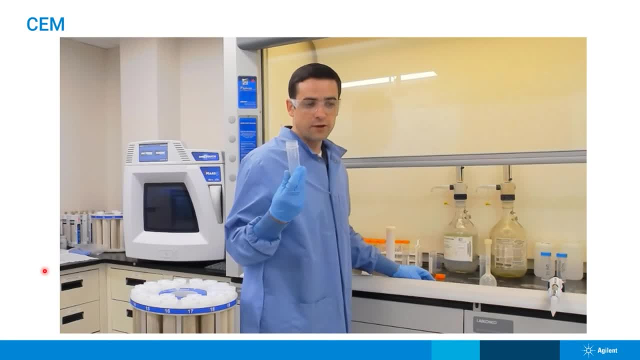 You want to make sure you pre-soak these containers and dilute maybe 10%- 5% nitric acid for a day or two before you use them, just to make sure they're clean, even though we're pretty sure it's. the ones we get are clean beforehand. 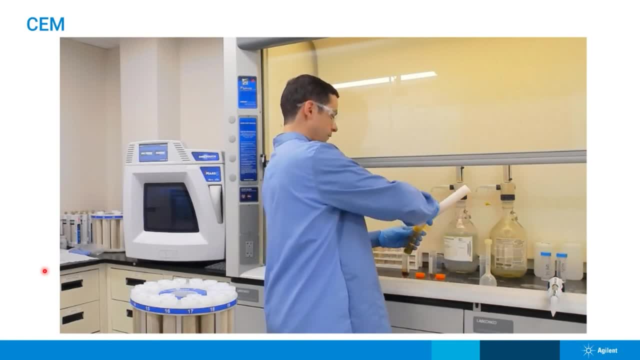 So you'll pour your sample into there and you want to quantitatively transfer. We typically do three rinses: out of the liner and into the centrifuge tube. So obviously you'll have this container pre-teared before you add anything to it. so 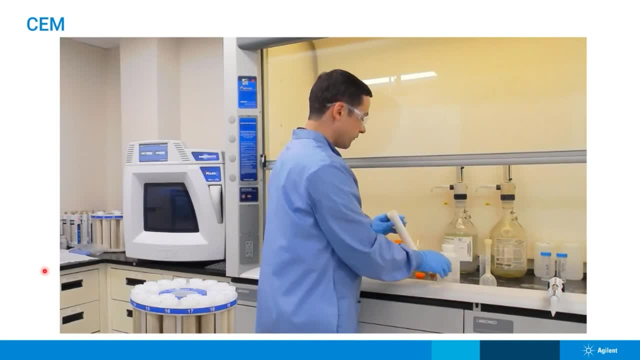 that you can dilute to weight. For our method, we diluted 50 mils using 10 mils of acid. You could get by again, though, with as little as 5 mils of acid, depending on your samples. All right, so three rinses just to make sure that we transfer everything, nothing's. 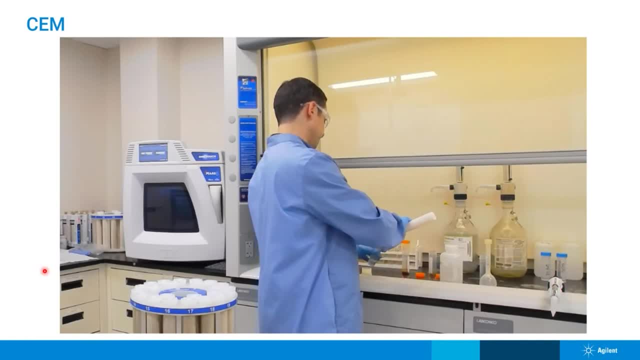 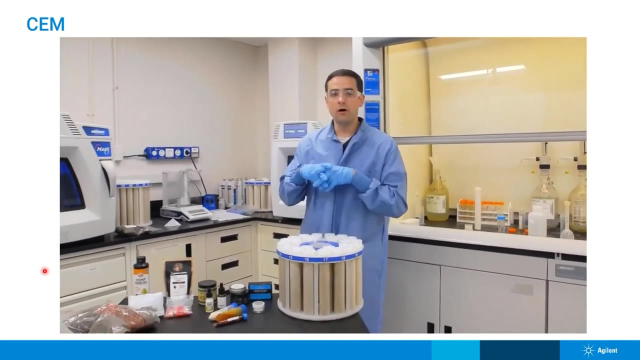 stuck to the side. You want to make sure that you get everything out of there, All right, and then we'll take it over to the balance and dilute to 50 grams, and we're done, All right. so to recap, you can run all of these different samples. 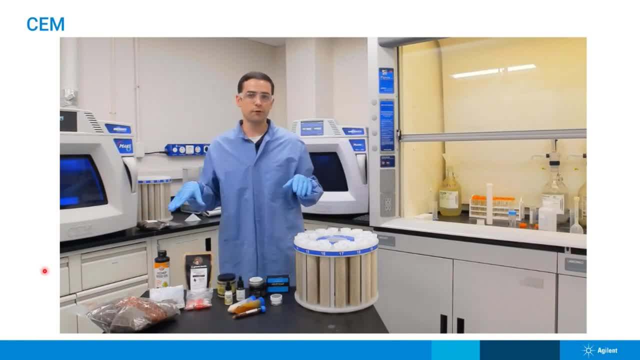 Our method encompasses all the different cannabis and cannabis-derived products, including the one I just showed you, Including, but not limited to, plant material, foods, beverages, consumer products and manufacturing intermediates. right, So you can do all of these different samples using our Mars Express Plus vessel set. 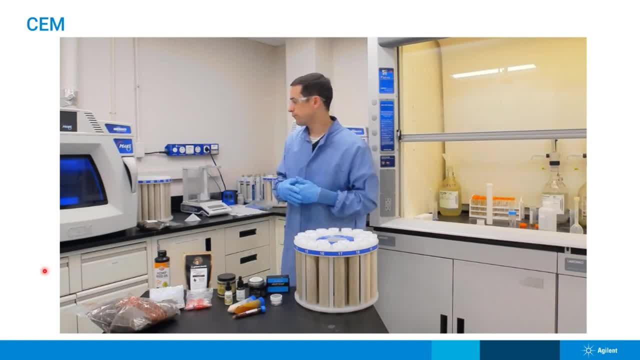 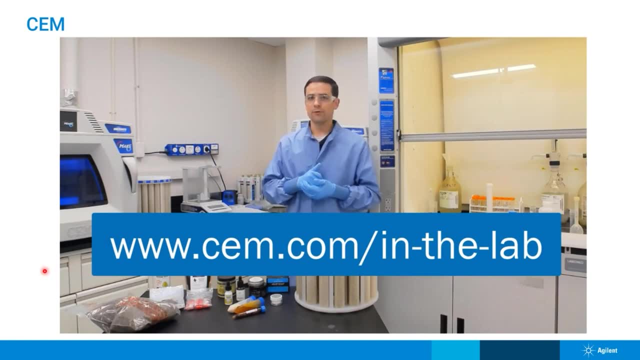 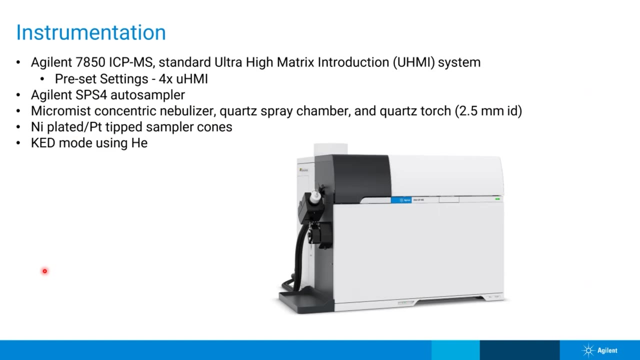 All right, if you want more tips and tricks on how to perhaps weigh your samples up, visit our cmcom in the lab for further tips and tricks, And I believe that's it. Okay, all right, so now that you know the microwave digestion and how we get the samples, 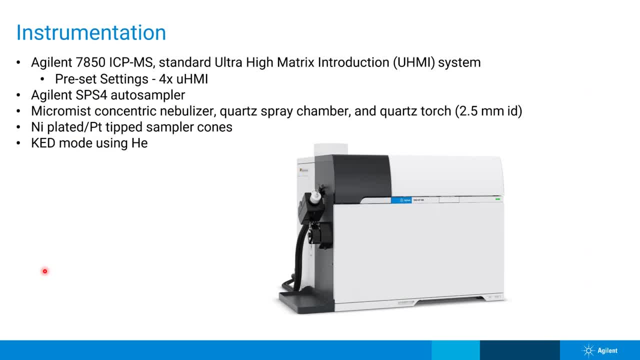 into solution which actually, to be honest with you, is really, really important, because if the samples aren't digested correctly or they're not digested cleanly, we are never going to be able to see those trace-level elements in the solution. 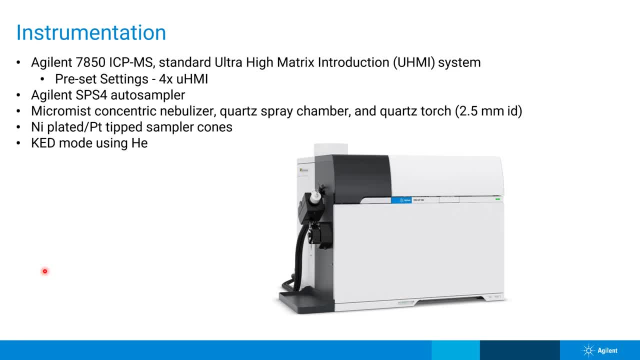 So you have to really follow the advice that the sample preparation people give So that you have clean acids, clean containers, because we're looking for parts per billion metals in these solutions. So you can imagine if you don't have a very clean setup and a good way to do the digestion. 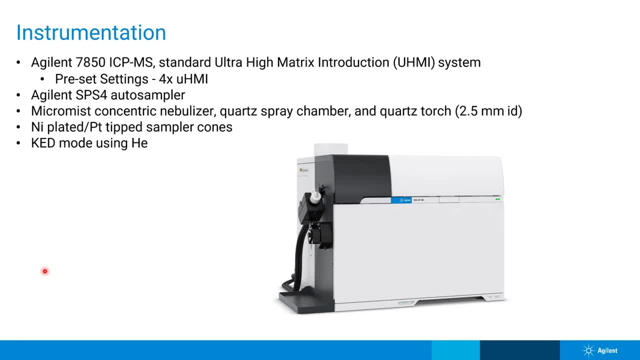 you're never going to see that low, So that I can't emphasize enough how important that side of the analysis is. So after you get those clean samples- or you know in a lot of people's labs they're doing it themselves- then we take it over to our ICP-MS. 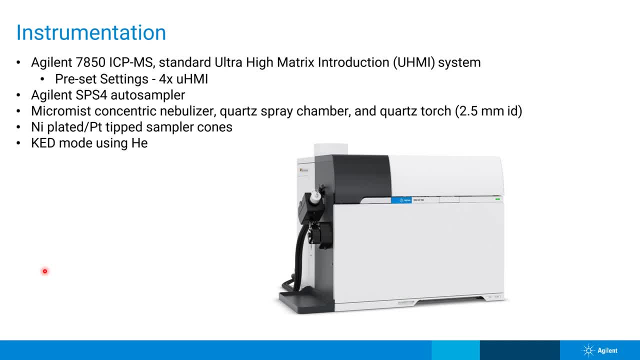 And, in our case, for our method development for the AOA sample analysis, we're going to do a single-quad ICP-MS And we're going to do a single-quad ICP-MS for the AOAC and the ASTM methods. 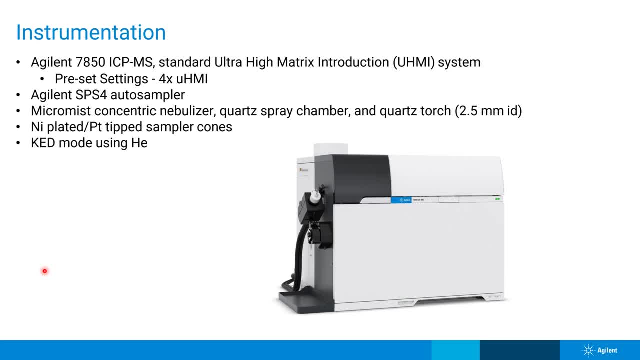 We used a single-quad ICP-MS. In this case it was an Agilent 7850 ICP-MS, which is our newest single-quad here at Agilent And since I work for Agilent, obviously we're using an Agilent instrument. 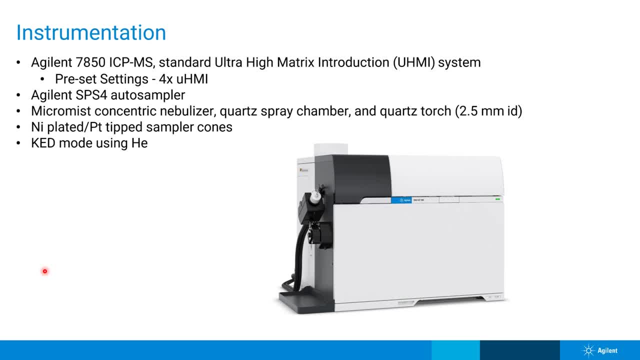 This instrument has a UHMI introduction system, So what that stands for is ultra-high matrix introduction And that allows us to run high matrices into the instrument, And you can see that for the cannabis-type samples, this is possible that you're going. 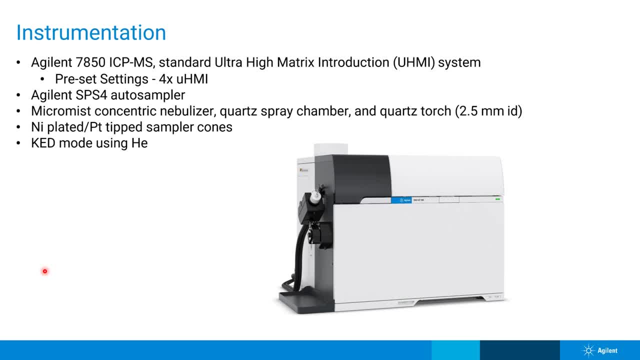 to have higher matrices versus some other things that you're running Like. if you're looking at drinking water, for example, that's a very low matrix thing that you're putting into the instrument. But if you're looking at, say, some of those crude extracts of the cannabis or some of 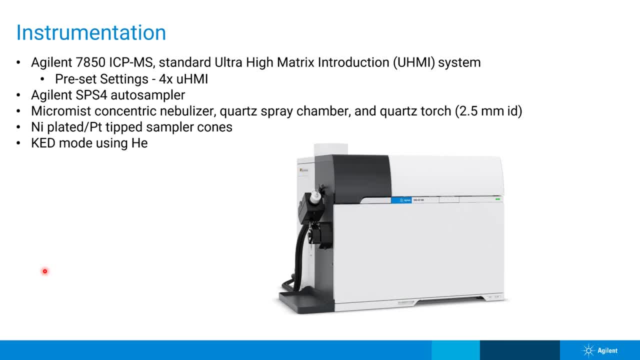 those isolates. you're going to have some pretty heavy matrices there And by using this instrument we're able to use preset settings. In our case, we used a 4X. This is the UHMI setting, so that we're able to run all the samples, all the different. 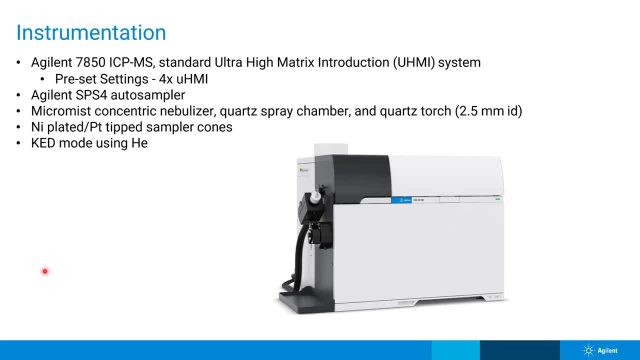 cannabis samples all in one run, So that's super helpful. We also just use the standard SPS-4 autosampler and then just a regular setup for everything else, like the nebulizer, the spray chamber, the torch, And then we use regular tones. 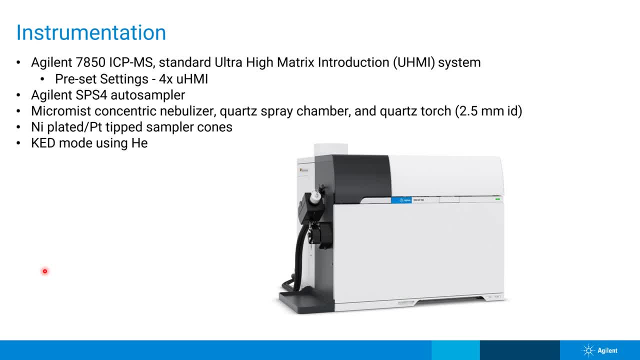 And then we use this thing called a collision reaction cell And I can show you this in a second when I stop sharing my screen. But we use a collision reaction cell, We use helium, We use helium gas in that collision reaction cell to do a kinetic energy discrimination. 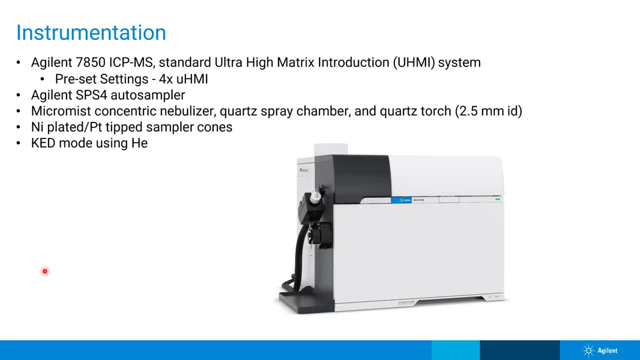 And what that does is it allows us to get rid of all of the polyatomic interferences that could be interfering with our elements of interest. So like arsenic, mercury, lead, cadmium, all of them, Okay, So here I'm showing you some of our 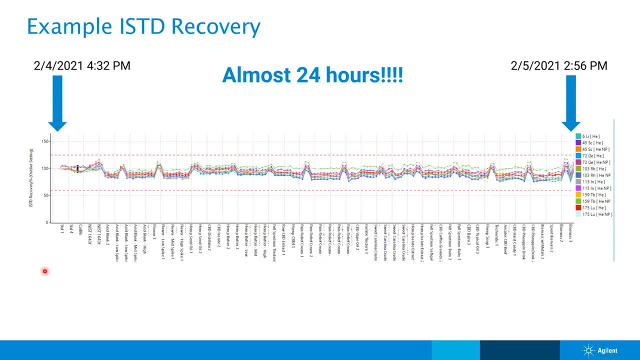 We're going to get into some of the data now. So this is an example of internal standard recovery. So we always T in an internal standard recovery So we know how the run is going throughout the course of the run And you can see this run was almost 24 hours long. 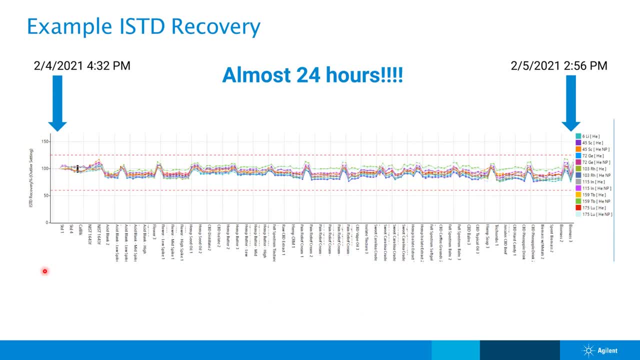 And we have really good internal standard recovery. So within the 60 to 120 range recovery of our internal standard. So the internal standards are elements that we're not looking for But again, we T in So we have a sample stream of our actual samples. 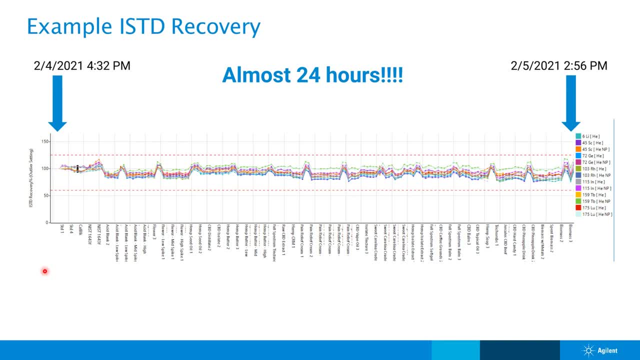 And then we have a sample stream of an internal standard And those mix in a mixing T and go to the instrument And some of the elements that are used for the internal standard you can see on the right-hand side here. So lithium, scandium, germanium, rhodium, indium. 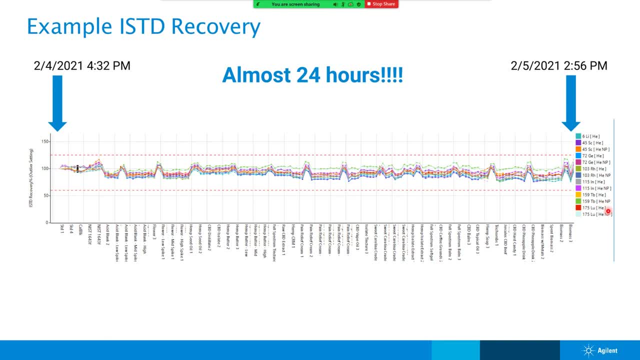 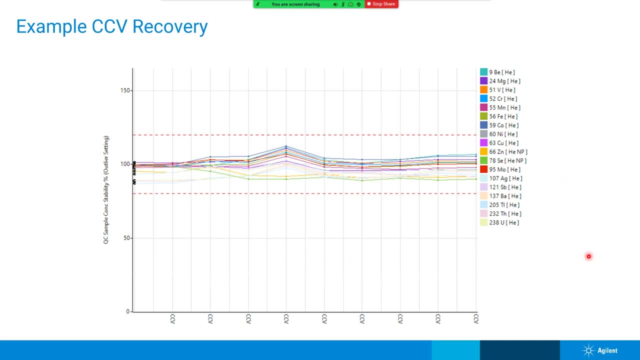 There's a whole bunch, And these are things that we're not going to find in the sample, Because you obviously can't have stuff that you're going to find in the sample be used as an internal standard. We also do a lot of QC in our method. 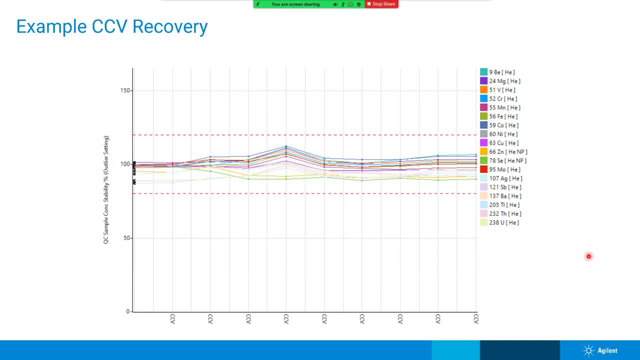 So this is an example of a CCV, So a continuing calibration, verification, And this is just showing some recovery, like within plus or minus 20 for the elements of interest. So these are elements that we're looking for in our method. 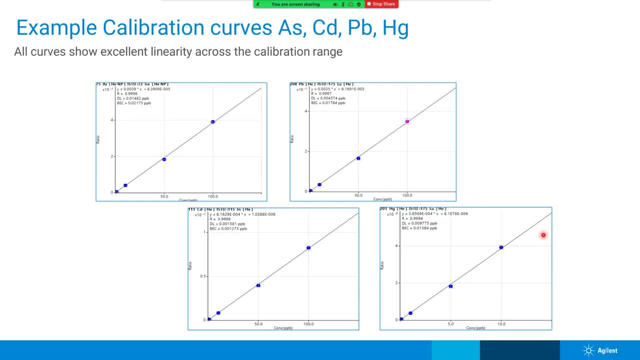 Here's just some examples of our calibration curve And so these are the big four- Arsenic, cadmium, lead and mercury- And you can see across the board we had really good linearity across the whole calibration range. And here's some examples of some of those optional elements in our method. 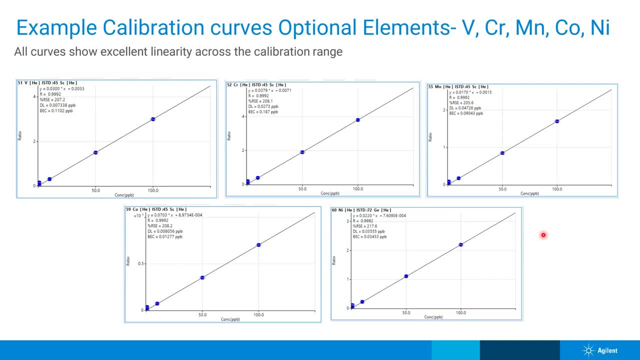 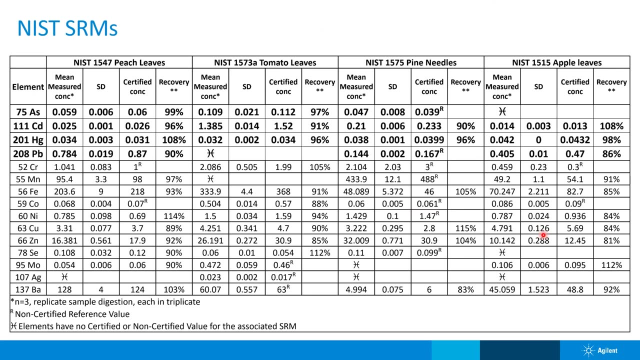 So vanadium, chromium, manganese, cobalt and nickel, All right, And obviously we have to run some SRMs And this is a part of the AOEC SMPR requirements. So we looked at four different SRMs. 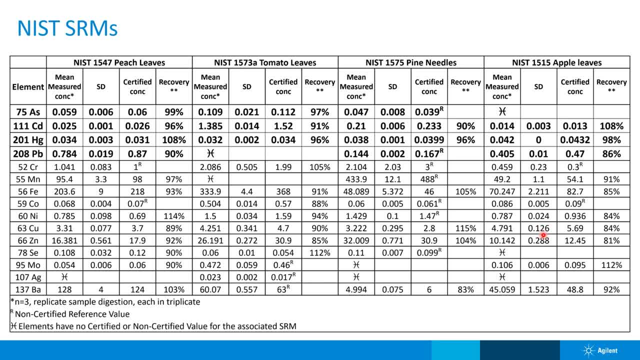 And at the time of doing the AOEC method development, there was no SRM standard reference materials for cannabis that were certified for metal, And so we had to use other products. So these are like plant life. These are the types of products that we could use as substitutes, because the matrix is pretty similar. 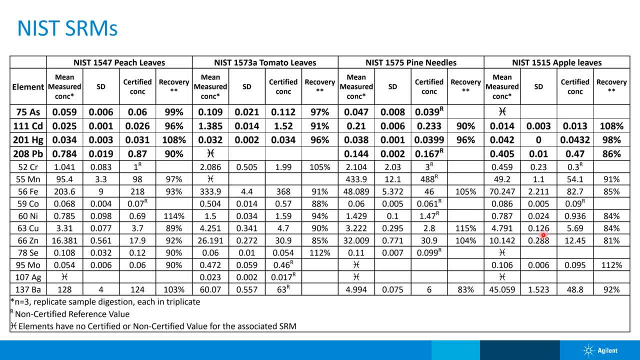 So these are food products or food-like plants. So we looked at peach leaves, tomato leaves, pine needles and apple leaves And across the board we were within the plus or minus 20% for the certified elements. Okay. 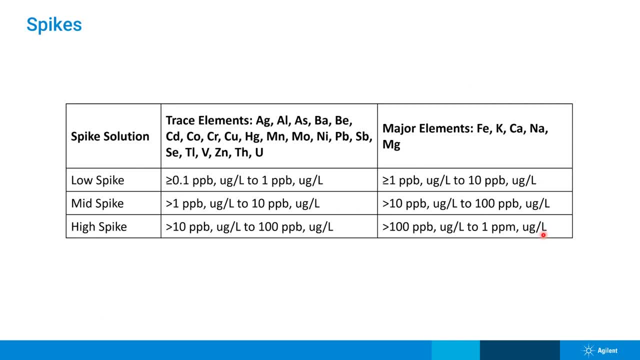 Another thing that we had to do to meet the SMPR requirements was to do spikes. So we had to look at each of those different categories. So there was the topical, oral, manufactured and flowers, And we had to do different spike levels. 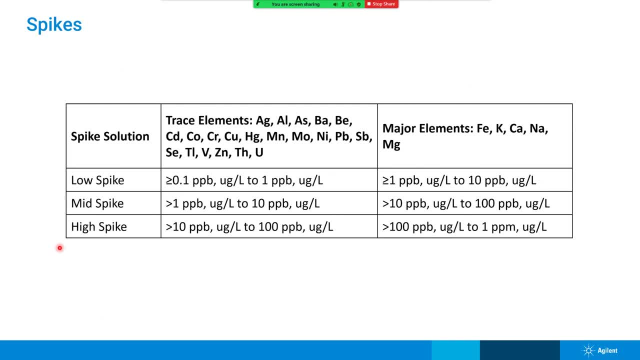 So three levels of spikes- low, medium and high spikes- for all the different elements and all the different matrices. So this was quite a lot of work And we had to do everything in at least triplicate. So this was lots of samples and lots of work. 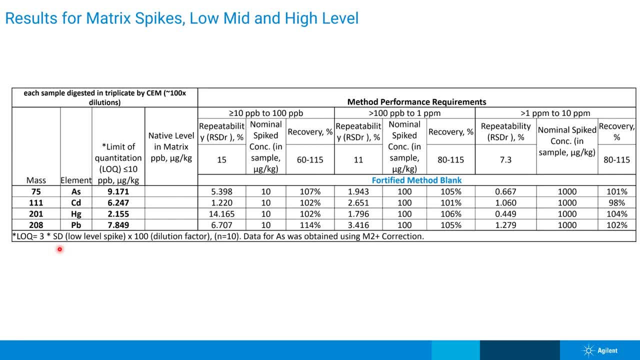 But here's a few of the results that I'll share with you, And I'm just going to share them with you. And I'm just going to share with you the big four, because this would just be an overwhelming table of data if we looked at all the elements at one time. 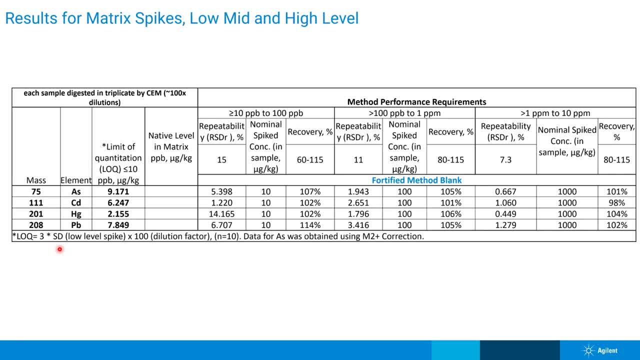 So this is a fortified method blank. So basically we're taking a blank through the whole digestion process, but with the spikes included for those four elements And across the board we met all the requirements that the SMPR set out for each of these different levels. 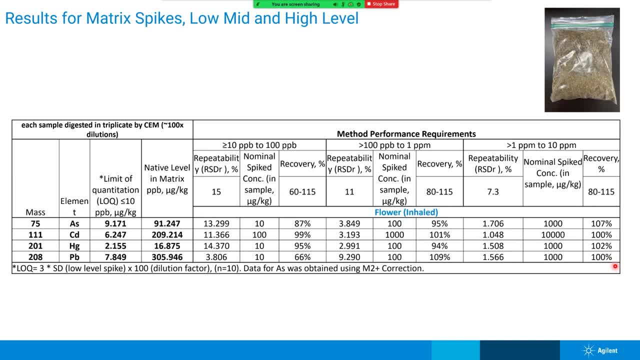 And this is the spikes for the low and medium. And this is the spikes for the low, medium and high levels. And this would be for the actual flour. This was for the cannabis product And we could meet all the spike requirements for recoveries and repeatability for this as well. 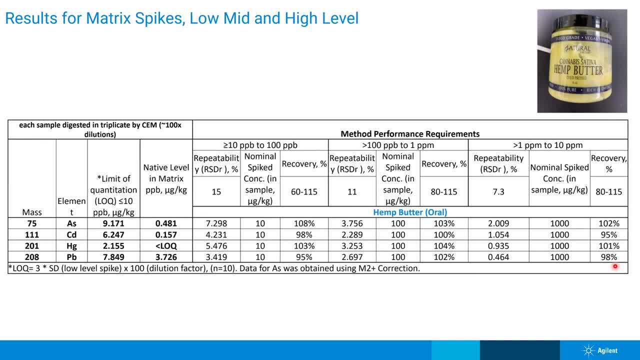 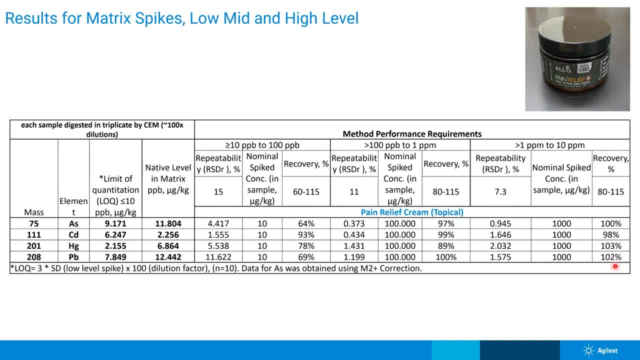 And next is the oral. So for this we used the hemp butter And we met the requirements. And this is the topical. So this was the pain-release cream And we met the requirements for this as well. And then the last category. 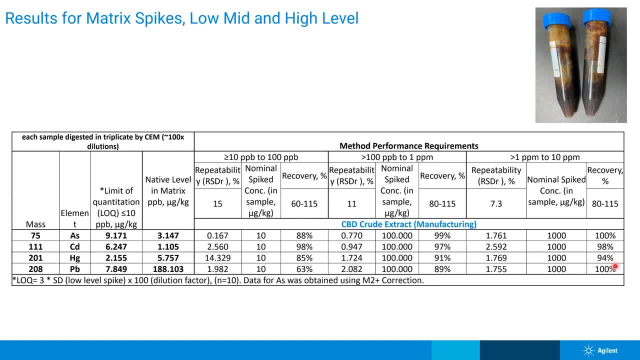 The last category was the manufactured products, And all the requirements were met for this as well, And so that was a big study And that took a lot of work, And Sam and I were both in the lab for a very long time to get that all done. 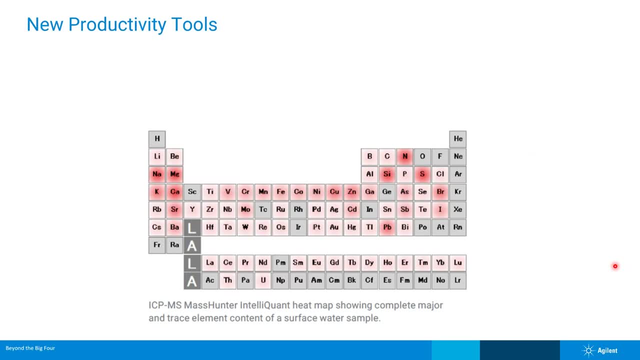 Okay. One thing that I wanted to add- that we have these capabilities with this instrumentation- is that we're able to do automated half-mass correction, And that's important, Because doubly charged ions can appear at half their mass And these can create errors in this type of analysis. 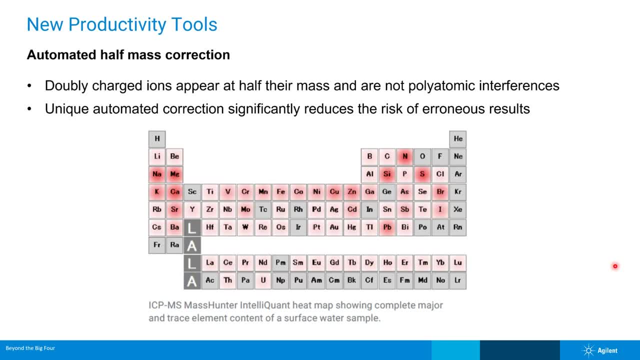 And this is important because, again, we're looking at plant material. Plant material is grown in the ground, And in the ground there's rare earth elements, And one of the elements that is one of the main elements that we're looking for is arsenic. 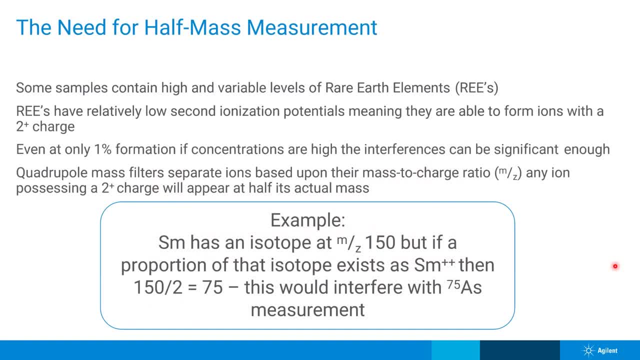 Okay, And arsenic is monoisotopic, So a lot of Well here. I always have this in my hand, So if you're not used to looking at the relative isotopic abundances of different elements, a lot of times when you're doing ICP-MS if something has an interference you can just go ahead and look at a different isotope. 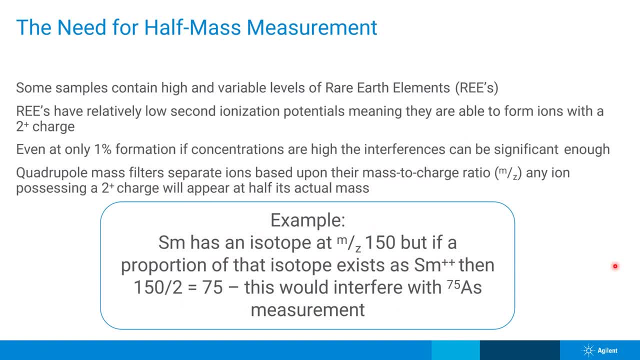 But if you're looking for arsenic, there's only one isotope- That's why we call it monoisotopic- And it has this problem that when there's possibility for rare earth elements to be in the sample, this can be an issue. 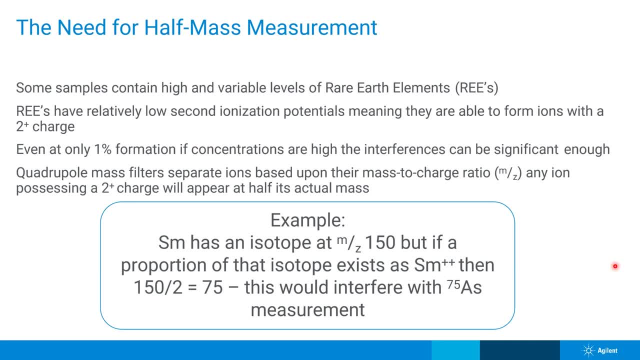 Because one of the rare earth elements is a samarium And samarium has a mass of 150. And because it can easily lose its second ion, so it can be doubly charged. 150 over 2 would equal 75,, which is right on the isotope for arsenic. 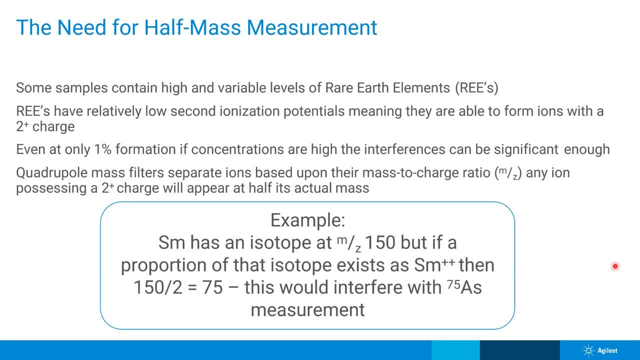 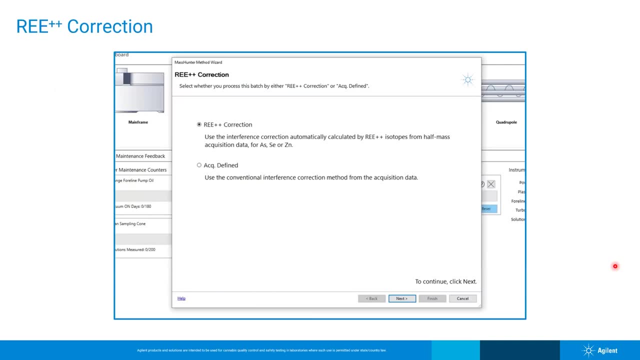 So you can see where this could be a problem for our analysis in cannabis- And I've measured a lot of cannabis samples and I definitely see rare earth elements in cannabis just because, again, it's grown in the ground. Okay, So with our software, we recently updated our software to this 5.1 mass hunter and we're now able to, just by a click of a button, be able to do corrections for those rare earth elements interferences. 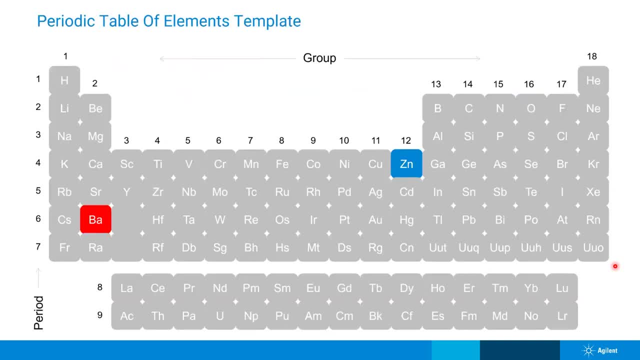 So that's good And we use that for this method, I should say. Another example would be for zinc, And zinc is one of those optional elements that a lot of people like to look for, And its doubly charged interference would be from barium, which is also a possibility to be in cannabis samples. 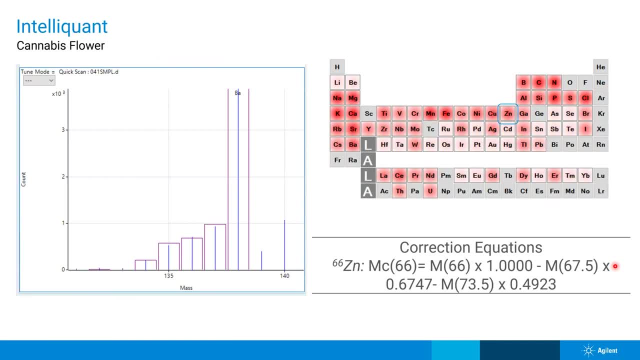 Okay, And you can see here this is one of the cannabis flowers that we were looking at. And just to confirm that barium was an issue, you can see I overlaid an isotopic template of what barium's isotopic template. 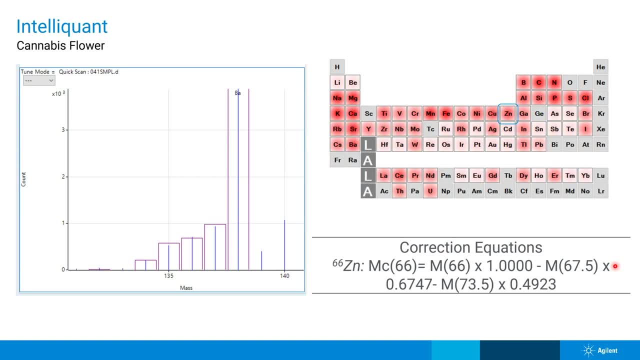 And you can see that this would cause an interference on zinc to give false results. So we're aware of this. We have obviously these rare earth element correction equations already automatic in our software And they're easily, just by a click of a button. 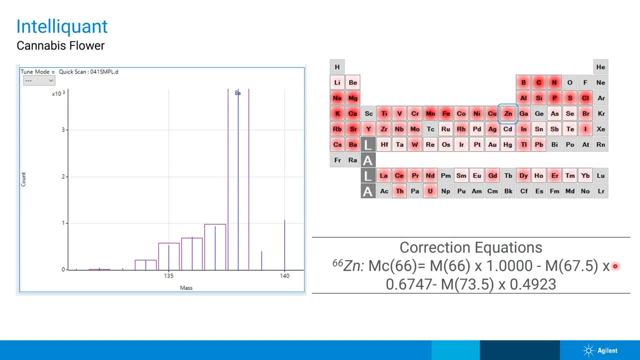 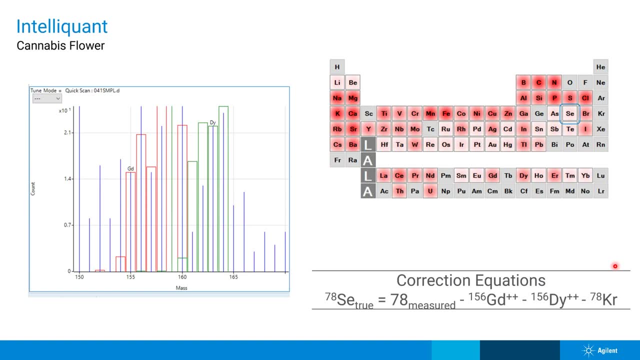 And so we're able to get around any of those interferences, So we can get correct results. Another feature- Oh no, This one is another example of looking at doubly charged interferences. Another one is for selenium. Another element of interest for cannabis folks. 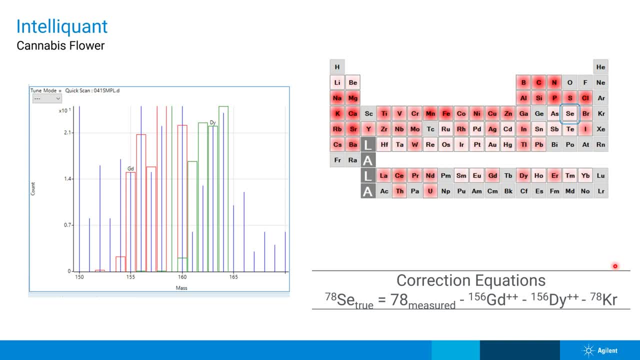 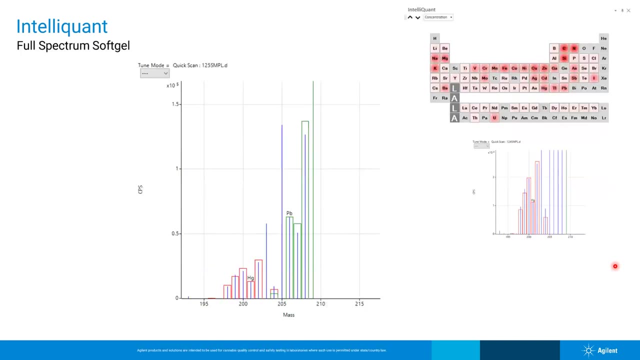 And if you have rare earth elements shown here, they can also cause a problem for selenium. But again, we are aware of this And our method deals with this And we have these correction equations already set up in the method. Okay, 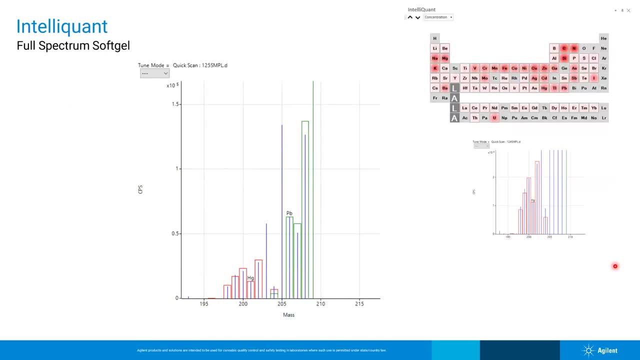 Another way that people like to use these isotopic templates is to actually confirm that some elements are in the sample, And in this case I'm showing you an isotopic template overlay of mercury and lead, And you can see that if someone was looking for just you know, one isotope of mercury, say 201,. 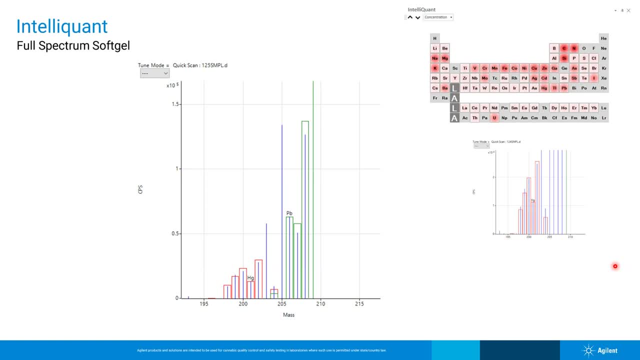 which is the common one that people want. Well, maybe if they just saw that one, they would want maybe more confirmation that mercury is actually there. Well, if you overlay the template, then you can see that you know all the isotopes for mercury are there. 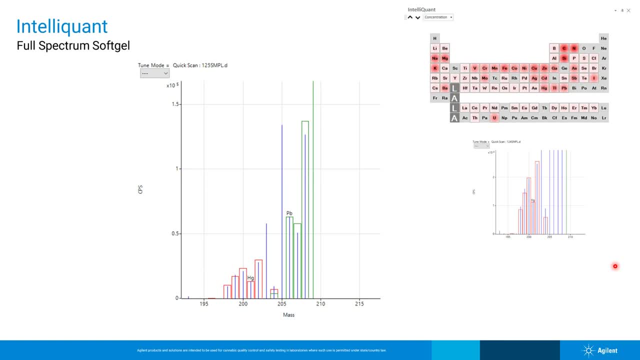 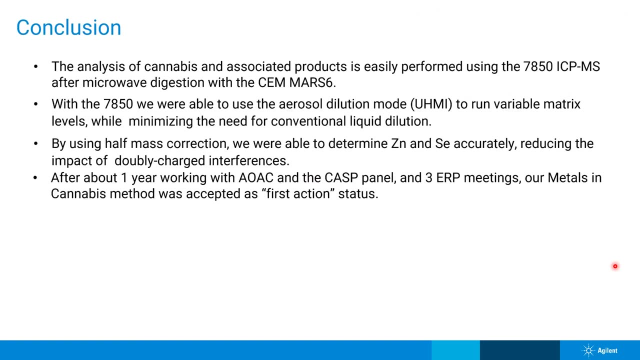 So you can be confident in the data that you're reporting. Okay, So in conclusion, for our method, by using the 7850 and the microwave digestion, we're able to successfully analyze cannabis And it's cannabis-derived products. We definitely utilize UHMI settings so that ultra-high matrix introduction setting, so that we're able to run a variety of different matrices. 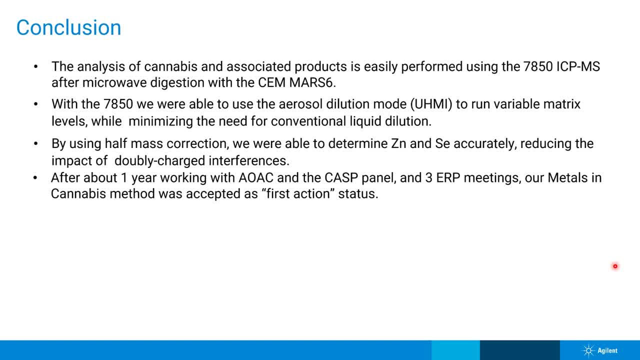 And we're able to use that half-mask correction so that we can correctly measure, you know, some of those elements that could have doubly charged interferences like zinc, selenium and arsenic, And after working with the AOEC and the CASP panel. so that's the cannabis group at AOEC. 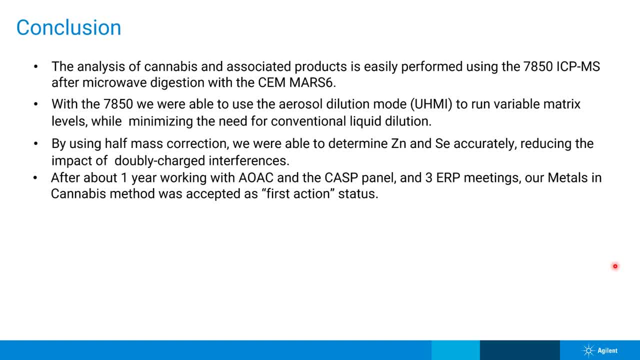 We had three expert review meetings. Our metals and cannabis method was actually accepted as a first action status, So now it's actually official. It's a first action status for AOEC And this was announced on August 3rd, And this is the OMA number. 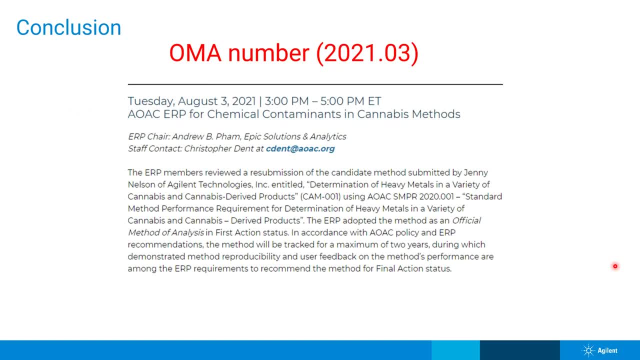 So this is the method number for AOEC. It's 2021.03.. And I believe it will be online through AOEC next week, I think Okay. So that's super helpful for the labs that are looking for some metal protocols in order to do their testing. 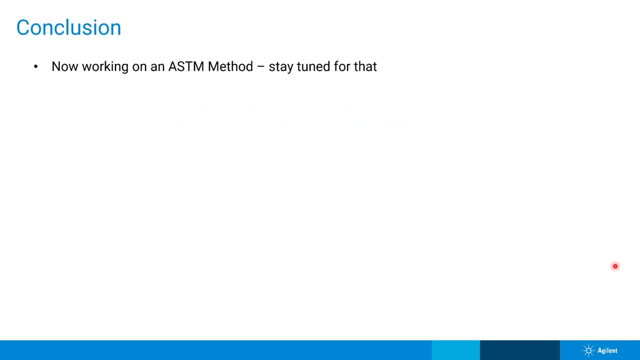 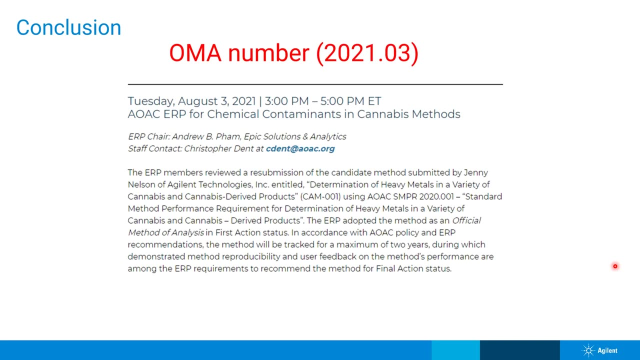 All right, Okay, So now that we have the – well, let me back up. So now that we have the AOEC – I'm going to back up to you this slide. Now that we have this first action, AOEC metals and cannabis method, we now have two years to complete an MLB, so multi-lab validation study. 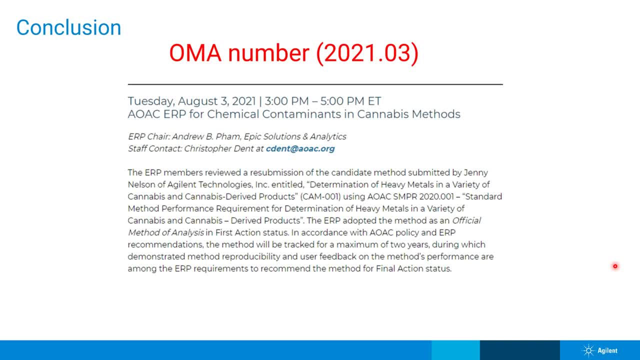 And so we're going to be looking to get a bunch of labs to do that with us using our method, And we are going to be working with NIST and some of their new SRMs that they're working on for cannabis, And so that's pretty exciting. 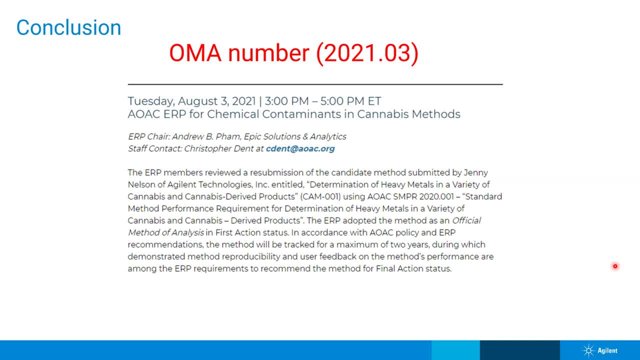 And that's going to be a pretty big undertaking, So we're excited to get into that. after this method is released through AOEC And Kyle, I'm going to reach out to you. Maybe you can join our MLB that we're going to be running. 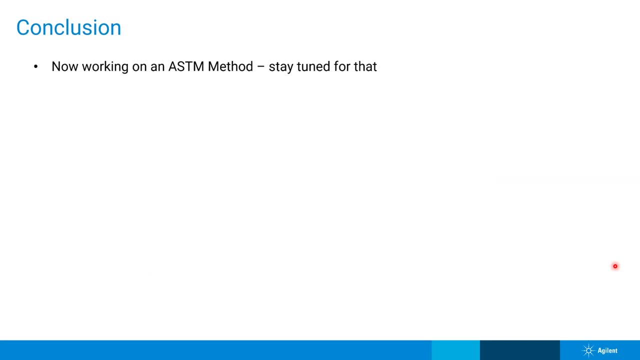 That we're going to be running soon. Yeah, we'd love to be a part of that. Oh good, And maybe some other folks that are on the call as well. they would want to be a part of our MLB study. So that's for AOEC. 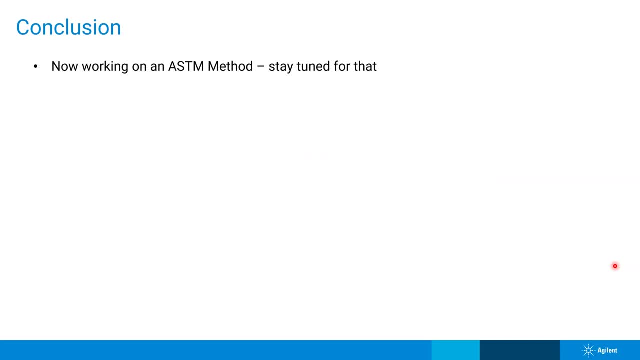 For ASTM. we are working on a method with them for metals and cannabis because we realized that, you know, not all labs follow AOEC and not all labs follow ASTM. So if we have a method- metals and cannabis method- with two different organizations, because you know we're going to be working with them, 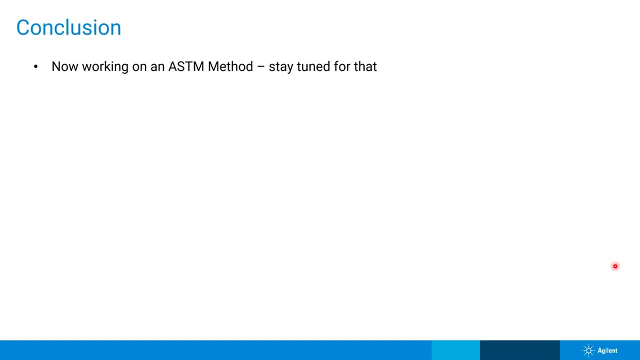 Okay, Different folks. depending on where they are in the world and what type of industry they're in, They could need to follow different regulatory bodies and different methods. So we are working with ASTM and we've written up a method for them And that will have to go to ballot. 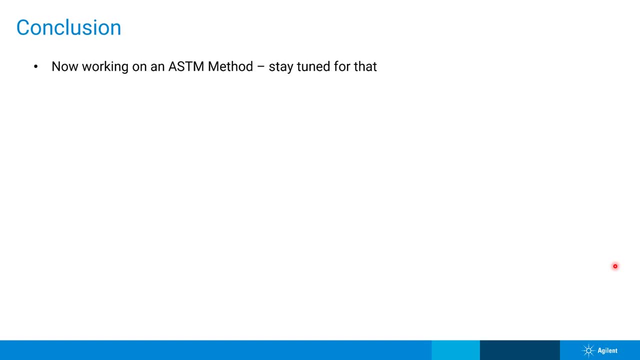 I'm not sure when, But it goes through a similar process where it's voted on and you know we have corrections to do, We have to meet with experts And it's quite an undertaking to get a method through One of these bodies.